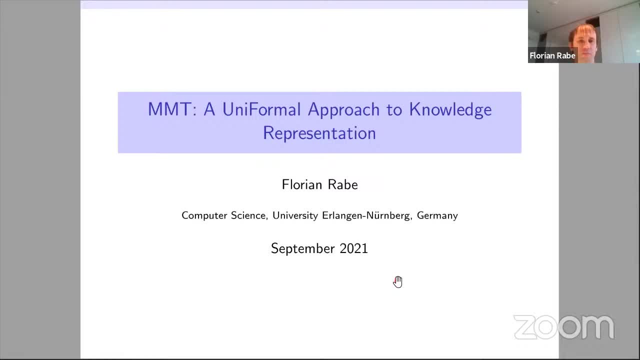 MMT is a system I built in my PhD thesis and that I have constantly refined ever since, And it has gradually taken over the entire research group. So nowadays, every student in the group is in one way or another working with the system. It's deliberately designed to be extremely flexible, So 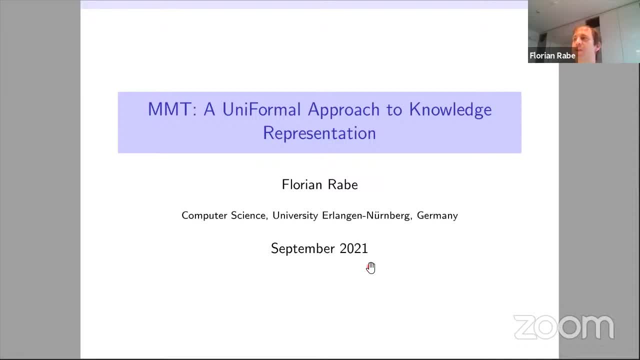 whatever interests the group develops, MMT is going to come in handy. It's a great system for rapid prototyping. so whatever one of our students wants to do, say, develop some domain, specific language, parse the material and send it to some theorem prover, then MMT is a great platform. 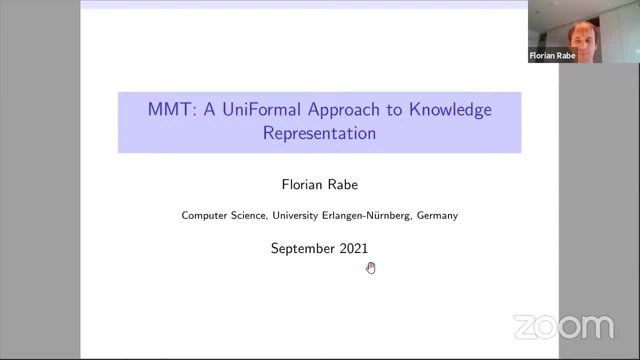 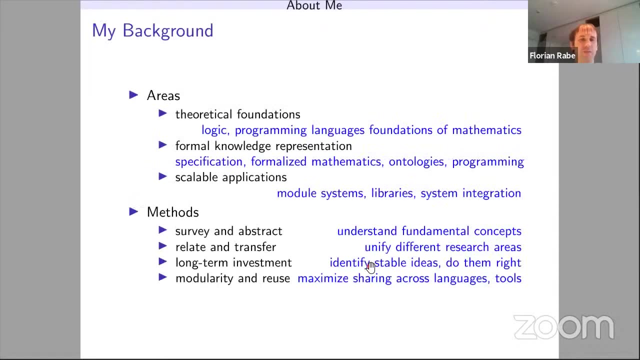 to put that together relatively easily. Let me tell you a little bit about myself before I dive into details. I'm mostly interested in your ideas, Thank you. In other words, I'm interested in your ideas in the theoretical foundations of computer science and mathematics, with particular interest in 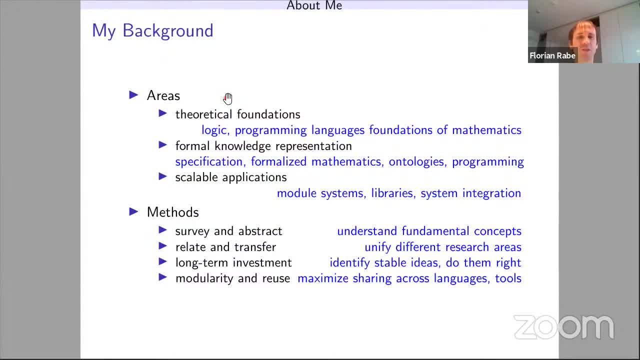 knowledge representation, And here I'm taking a very wide view. I'm interested in any kind of knowledge that can be formalized. So languages for formalized mathematics to me have the same status as programming languages, specification languages, ontology languages. 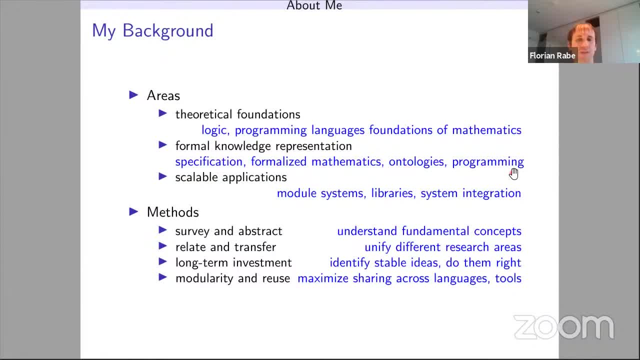 They're all just formal knowledge, representation languages, And MNT is built with the long-term goal of integrating all of those and supporting all of those in one system. I'm interested not only in the foundations but also in developing applications, mostly from the perspective of how can we build large libraries of formalized knowledge. 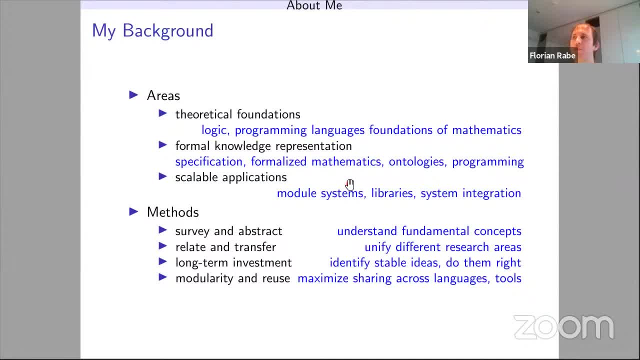 It's usually a huge difference between coming up with a prototype implementation and actually seeing how to implement it. I'm interested in supporting large-scale development in that language And, from a perspective of system integration, especially when you take such a wide view of languages, you're never going to be able to support everything in one system. 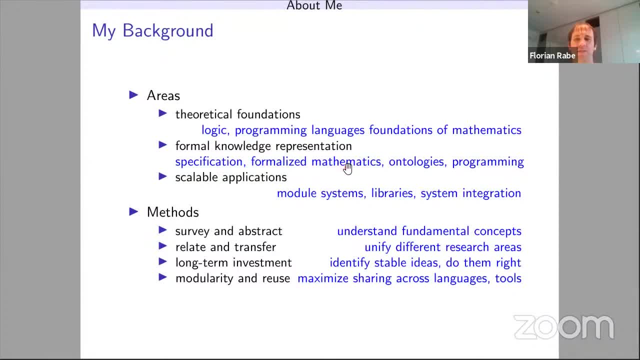 So you need to seriously think about how can you make very disparate systems work together in some reasonable way. I tend to focus on breadth of methods, So I love abstracting from various systems that are doing different things but applying similar methods. So like a theorem prover and a compiler, what do they have in common and what kind of generic? 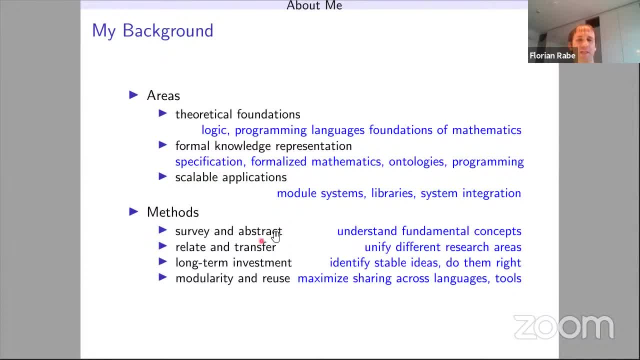 concepts can we extract from there that we can then integrate into MNT as some kind of universal knowledge representation framework? Generally MNT does not strive to make the individual as individual systems obsolete. So MNT cannot compete with any particular theorem prover. 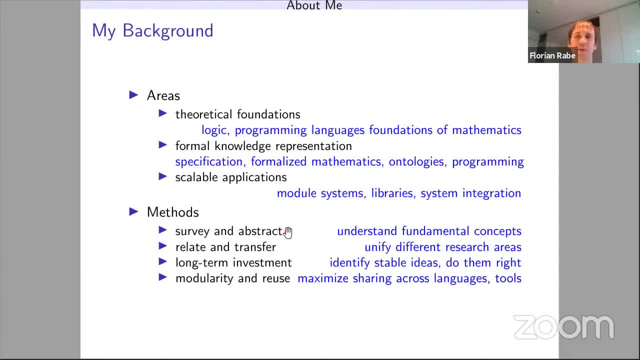 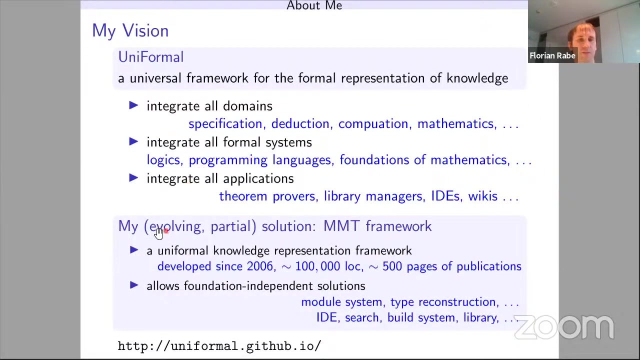 Those are usually heavily optimized to prove stuff about one specific logic. Similarly, it can't represent any particular optimized compiler which is heavily optimized to one particular programming language. It's meant to focus on the overall joint concepts that all these languages share. So we're calling this general goal uniformal, like one universal framework. 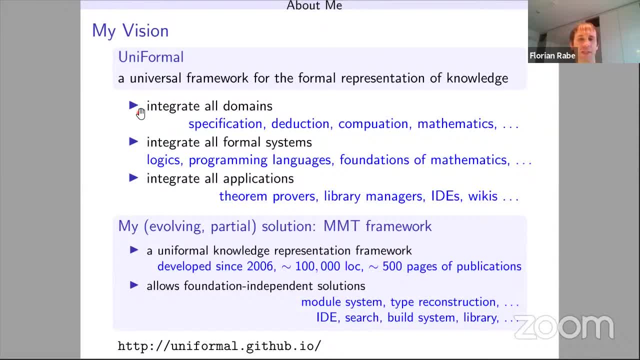 for all kinds of formal knowledge. MNT is by no means a solution to that problem. It's more like a moving target. It's whatever we've understood we capture in MNT, Either it's a conceptual or its implementation level. So it keeps evolving and responds. 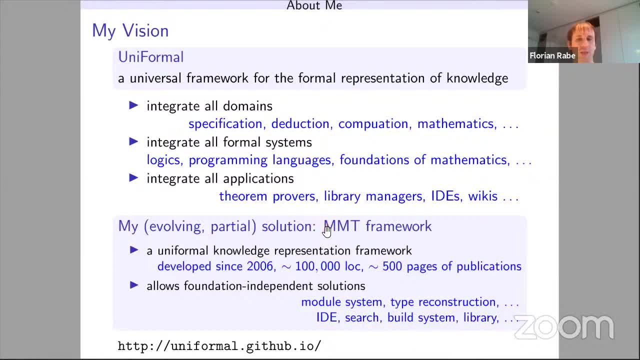 to whatever challenges we uncover. It's become quite mature by now And it has relatively strong concrete applications that allow, for example, make it as easy as possible to prototype a new logic and then get, say, a type reconstruction engine as an IDE out of something. So, for example, it's very easy for us to prototype a new logic and then get, say, a type reconstruction engine as an IDE out of something. 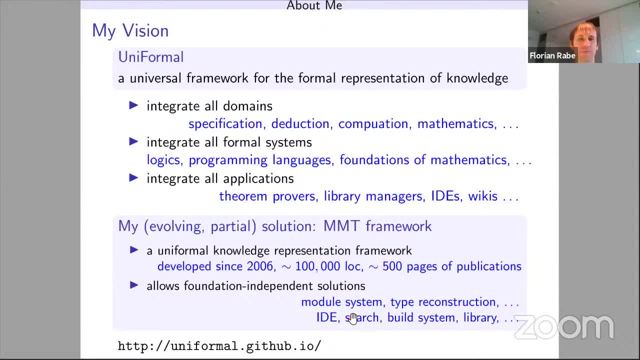 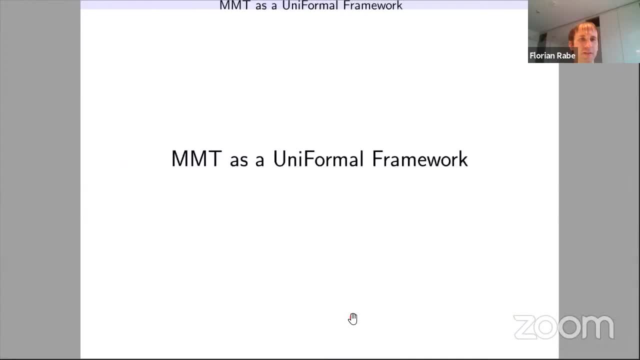 there's a box for that system. Skip these slides. I think I should say right away that I have a lot more slides than I can fit in one hour, So I strongly encourage you to ask questions to guide the talk into the direction you like. 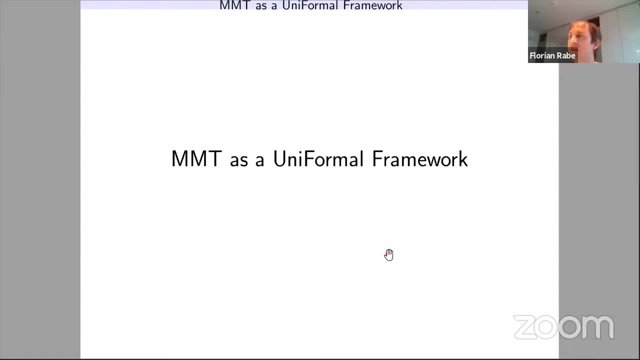 in particular when it comes to the trade-off between showing your nitty-gritty details about the syntax and semantics of MMT versus showcasing individual applications. So, depending on what you're interested in, if you want to see the grammar and the type system, I have slides for that. 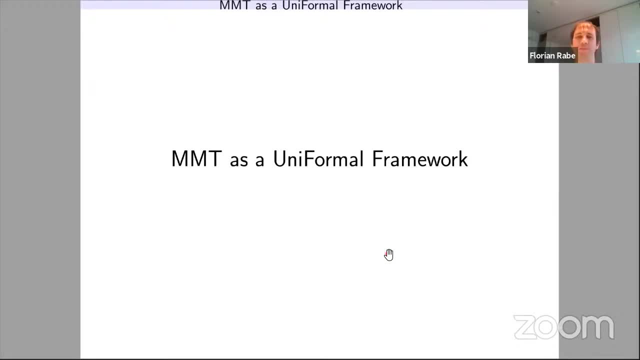 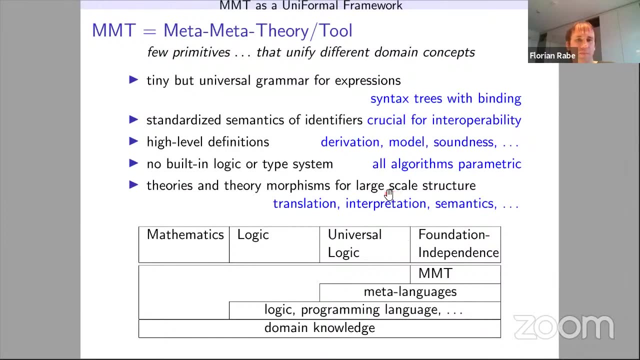 If you want to see screenshots and demos, I have examples on that as well. One more overview of this slide. So the idea of MMT is It can be best understood with this four-level hierarchy. The thing you're usually interested in is the actual domain: knowledge. 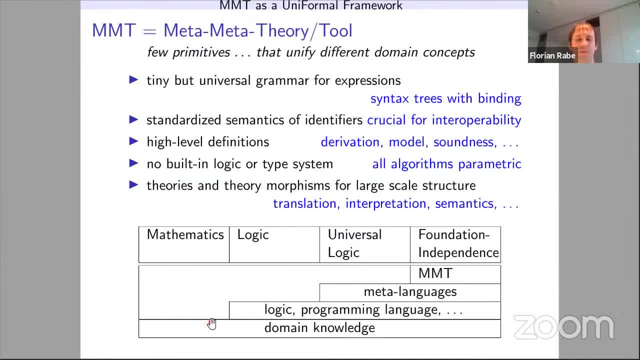 That's why mathematics is working basically exclusively. Then if you want to put that in a more formal setting, you have to invent a logic or some other formal language in which you write down your knowledge. Then you quickly find out that you end up with lots of different. 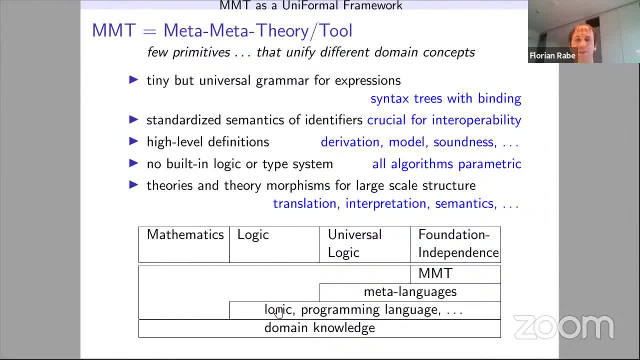 Logics or similar languages, like just first-order logic, higher-order logic, moda logic, already explodes at the logic level, And that's kind of my home area, That's where my PhD was centered. So you have all these different logics and you realize how can we relate them. 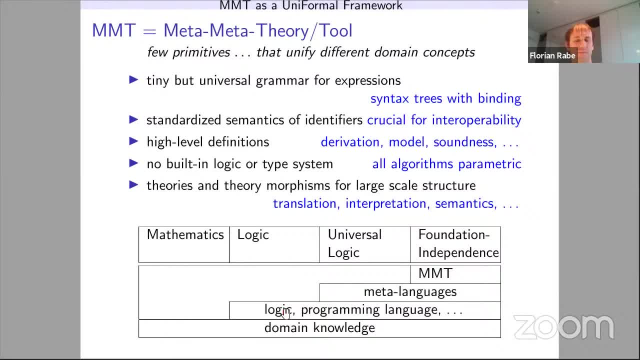 How can we get some structure into this zoo of different systems? So you have to introduce meta-languages in which you write down the individual logics, where you can then relate the logics to each other, Maybe do things in a different way. 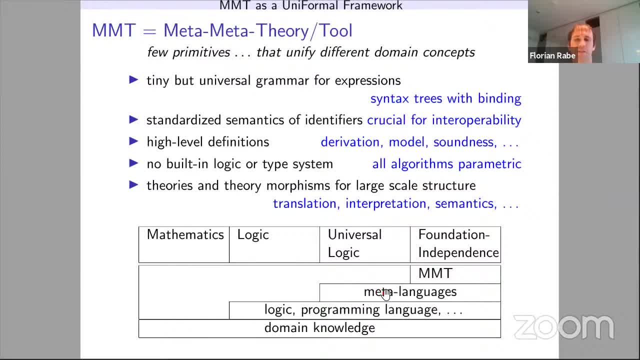 Maybe do things like logic translations or representation theorems across languages. In the area of logic, these meta-languages are usually called logical frameworks. The system I've worked with most is the LF family of frameworks. Maybe you've heard of the 12th implementation, but they all work very similarly. 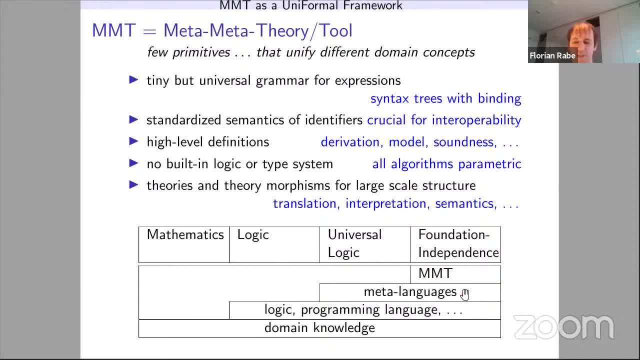 You pick one particularly simple, formal system in which you then present the syntax and semantics of the actual logical systems you want to work with. But even there we're struggling. First of all, well, the main problem with logical frameworks is that usually you want: 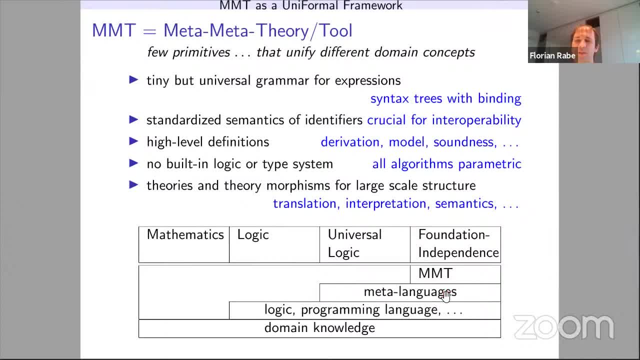 these languages here to be extremely simple, to justify their existence as, like, the one and only meta-language, But you also need them to be extremely expressive so that you can then represent all the various concrete languages you're actually interested in working with, And you see, this is very interesting. 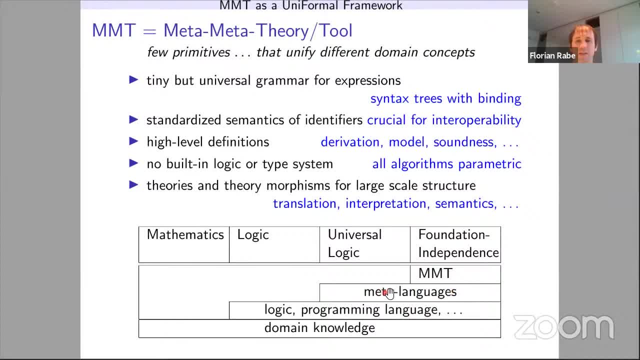 And I wanted to talk about this a little bit- And that's because we've got a lot of technical stuff going on And, yeah, there's a lot of stuff that's going on in the world right now, And here the state of the art is not really satisfactory yet. 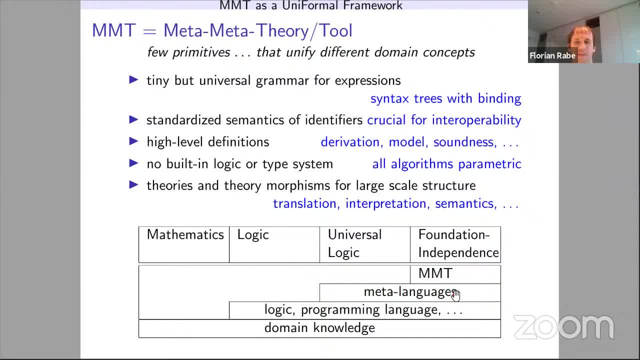 We have very nice logical frameworks, but they just can't represent all the logics that we need in practice. So we're constantly doing research about how we can improve our frameworks, And that means we constantly need to implement new frameworks, And that's where the idea of MMT came in. 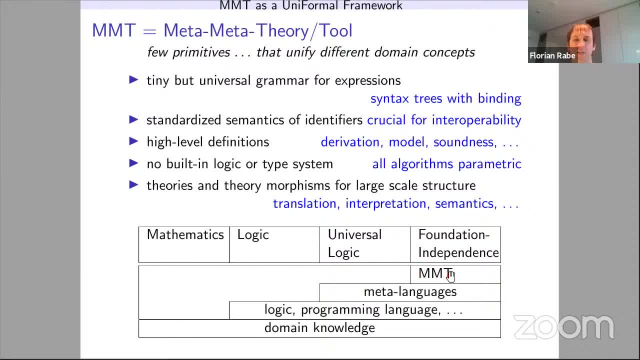 I wanted to implement my own logical framework, but I didn't really know which system that actually is yet. So I asked myself: can I implement as much as possible without committing to the concrete format system I'm working with? If you think about how people implement format systems, 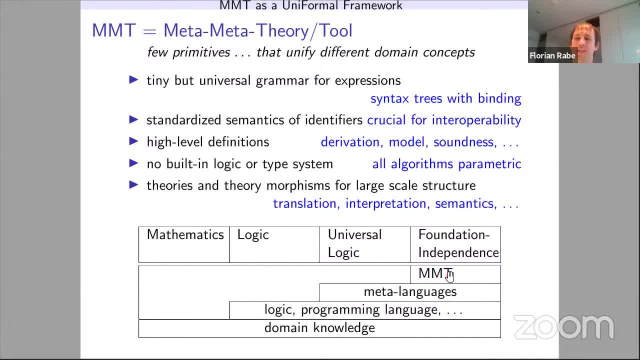 they usually start with a grammar and a type system, Then they implement a parser and a type checker for those. Then they build stuff on top like an IDE module system and so on, Which means the fundamental choices of which language you're working with. 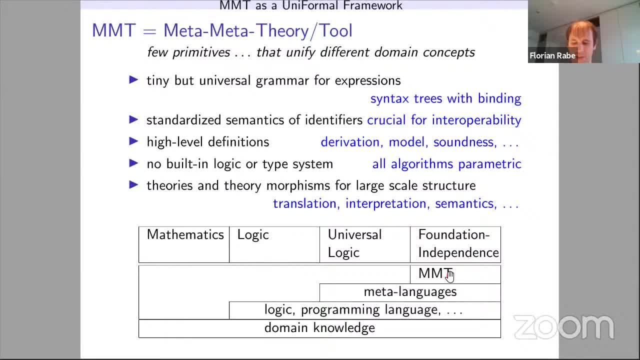 are baked so deep into the system. if you later on decide you want to change your fundamental language a bit, add a new kind of type operator or something like that, most of the time you're stuck because it's just not parsed anymore. 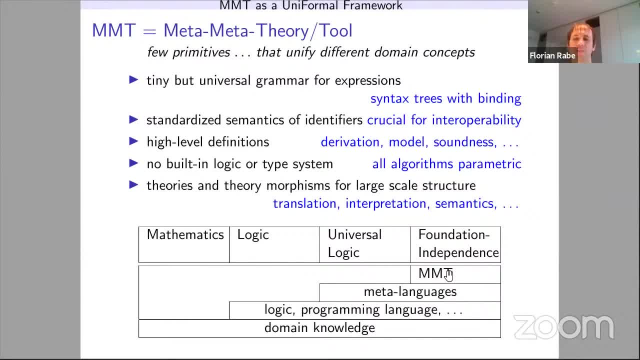 You have to change so much code, you just can't do it, or it becomes a huge undertaking. Just because you can't do it, it becomes a huge undertaking. Just because you can't do it, it becomes a huge undertaking. Just because you can't do it, it becomes a huge undertaking. 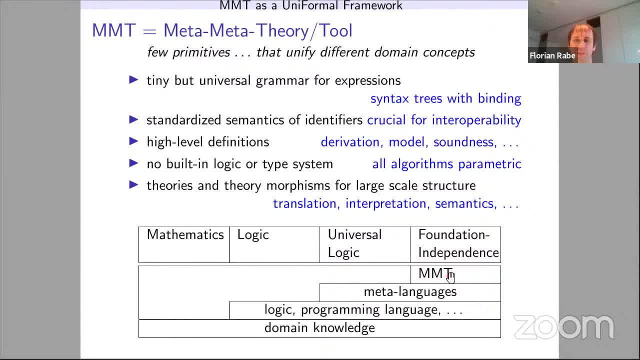 Just to add features to your system. So MMT tries to turn that inside out. leave the concrete choice of format system open and implement everything else. In the beginning that was just a research experiment. The question was: how much can we actually implement without committing? 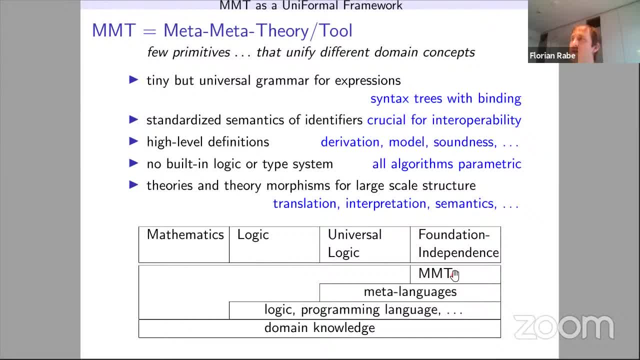 to the precise format system we're working with And in my experience that often has been up to 90% If you think about the implementation work of a specific logic you've come up with. usually parser and type checker are relatively easy to do. 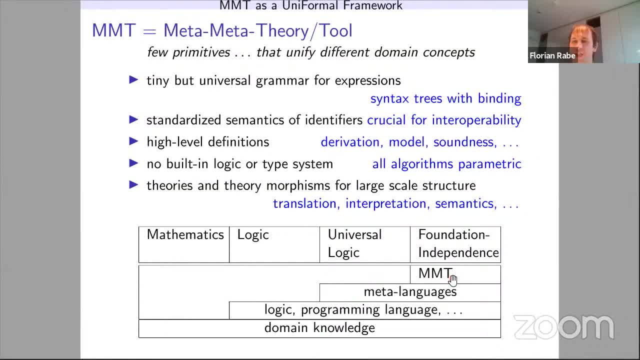 and then you have to write a lot of code to have nice concrete syntax, to have an IDE, a module system, eventually, of course, then theorem provers, computation engines and so on, But it turns out most of the work here. 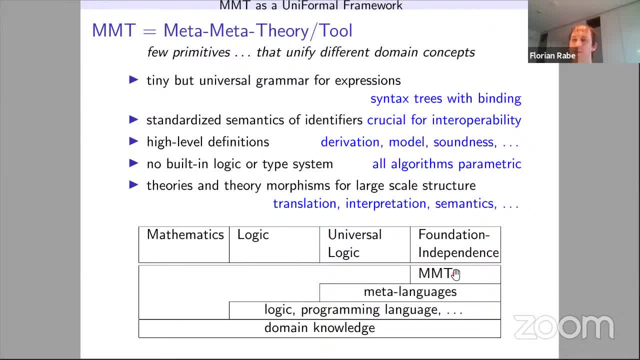 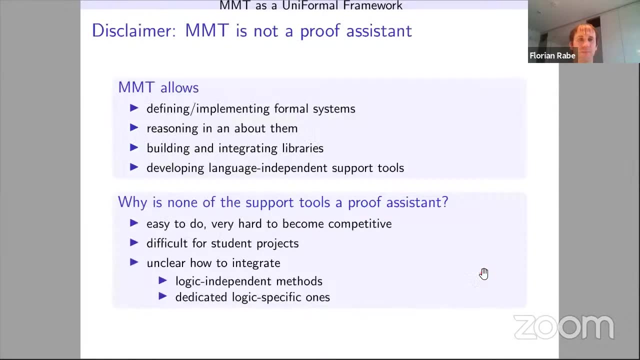 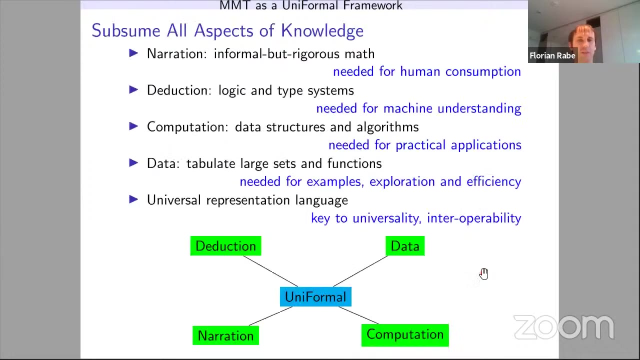 it doesn't actually depend on the logic. So the idea of MMT is implement all the algorithms generically and then later on inject the right rules to get the system you want. And before I go into the details, I have one more concrete slide of an essay. 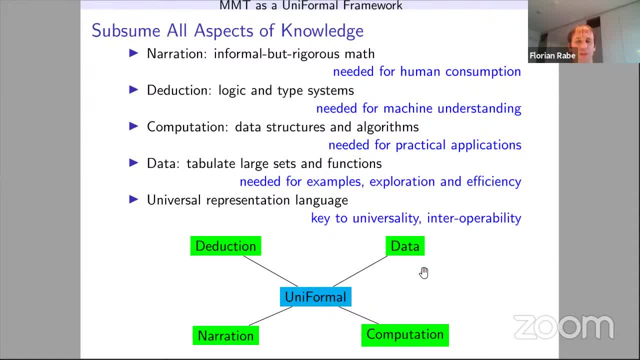 What I mean is when I say all knowledge. we've recently come to understand knowledge as a kind of- we call it the tetrapolar structure of knowledge, where we have four different kinds of knowledge. So here we have all the logical languages. 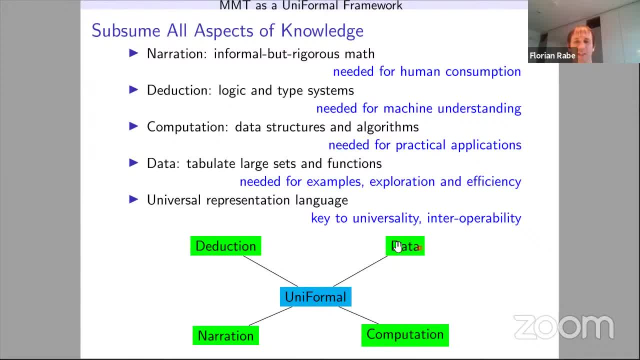 here all the programming languages, data representation languages which, especially in mathematics, are becoming more and more important, and natural languages in which we write down, especially in mathematics, a lot of content. So MMT is meant to sit in the middle of these. 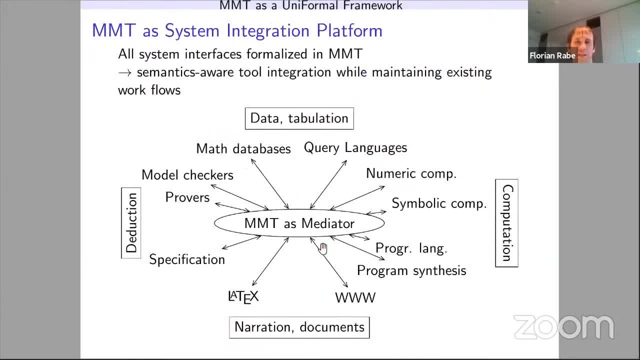 covering them all equally and allowing the interoperability across the different systems. Which means MMT mostly focuses on representing the joint essence of these four different extremes of how we can deal with knowledge. So MMT doesn't strive to be a theorem prover. 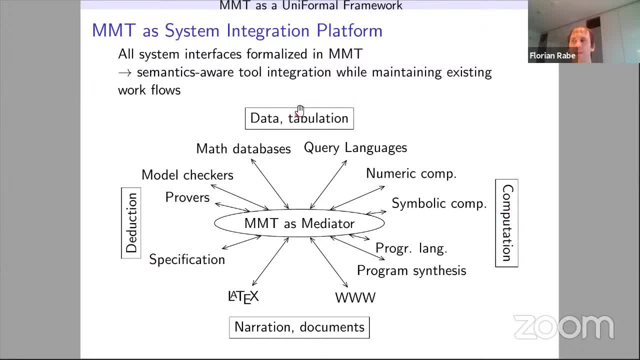 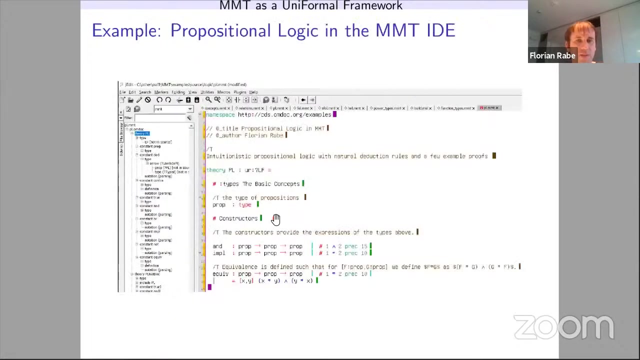 it doesn't strive to be a compiler or a database engine. It focuses on representing the common concepts, the ontologies, the data types which then allow mediating between the different systems. I want to start with some concrete examples. This is a screenshot from the MMT IDE. 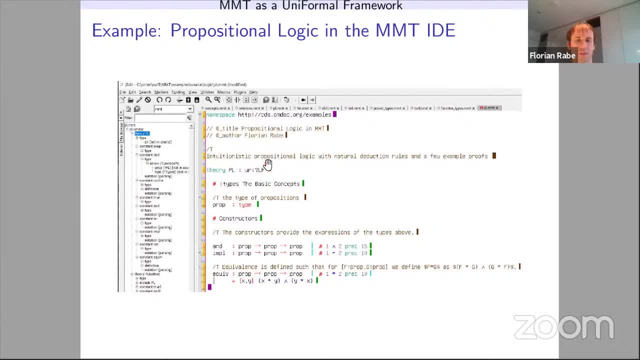 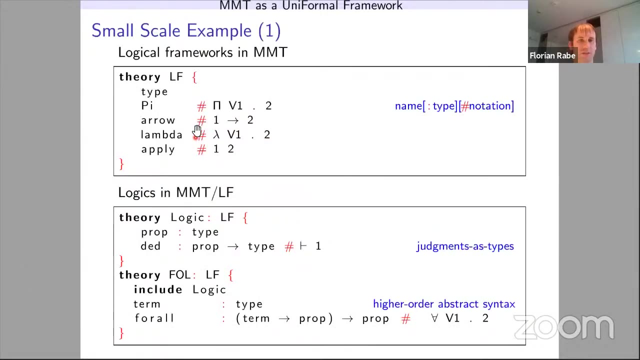 showing you a hello world. formalization of propositional logic using the logical framework LF. This screenshot is just to prove that the implementation exists. It's didactically better to show you a slightly more readable example. So I talked about the three layers before. 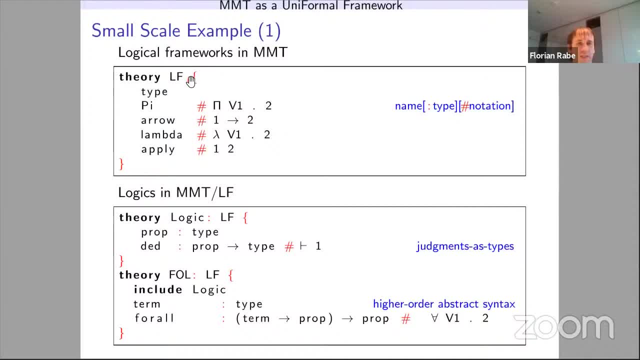 domain knowledge, logic, logical framework and on top of that, MMT. So that's what we are formalizing now. We start with a logical framework, in this case LF. We were presenting it as a theory in MMT. 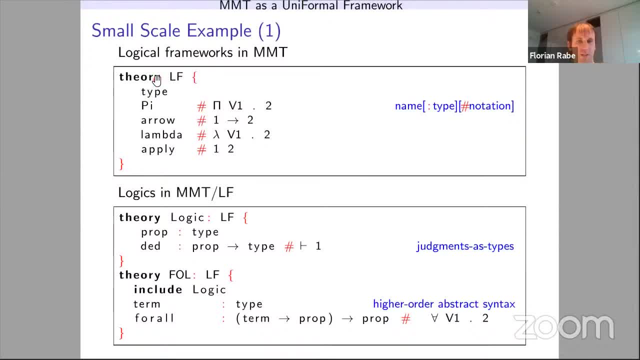 The word theory is often called signature. in other systems it's basically described as the name, the fundamental constants of the language. So in the case of LF, that's a dependently typed lambda calculus, we have the universe of all types, the pi operator, to build dependent. 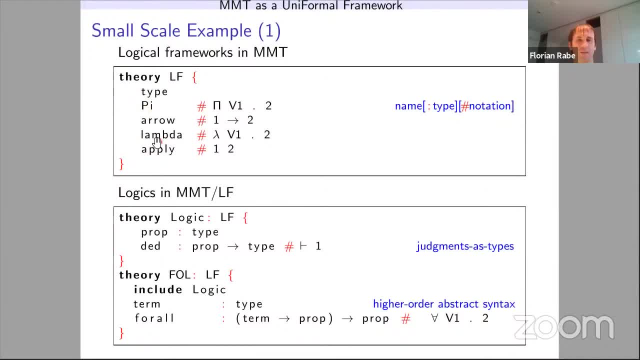 function types and the lambda and the apply operator to work with that type. NMT constants inside the theory are declared in the simplest case as name with optional type and optional notation. In this case, to get off the ground, we have constants that are declared. 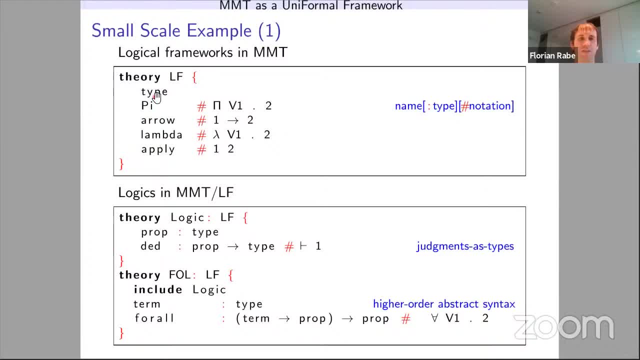 without any type whatsoever, because we don't have any syntactic material yet that we could use to form types. So the only thing we do is we give them notations, at which point we already have a parser and abstract syntax trees for our language. 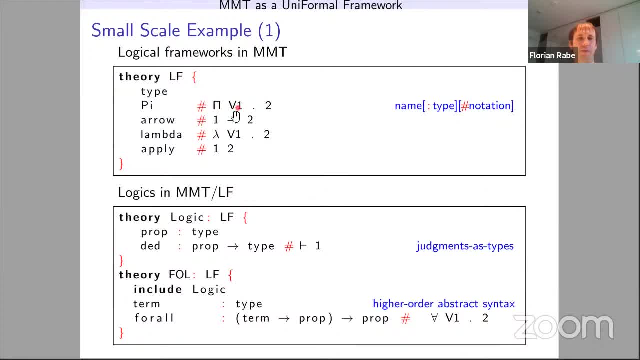 So this is the normal pi and lambda notations. V is for variable, which means this position is a binding. Of course we still need the semantics of LF. I can get to that later. That's where we have to inject RUIDs into MMT that implement the semantics of LF. 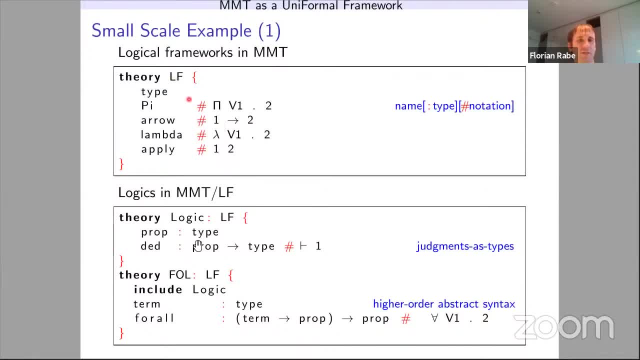 But let's assume we've done that already. then we can use LF as what we call a meta-theory to define concrete logics. So in this case we're defining some base theory that all logics can inherit from using LF as the logical framework in which it is written. Now we can declare a type of propositions. 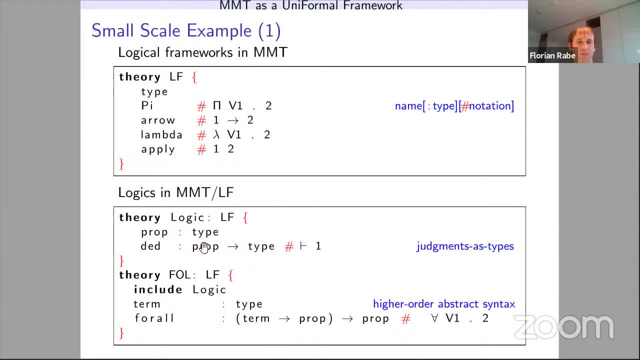 and a type of deductions for every proposition. So let's use a judgment of types paradigm where that F is the type of proofs of F. We can then extend this base theory by including it and defining other logics, such as first-order logic, where we might add something like a type of terms. 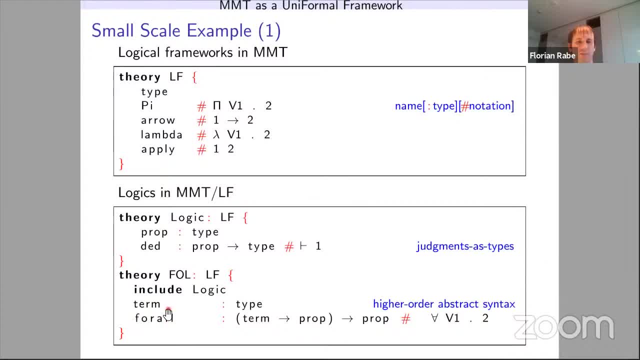 and then a universal quantifier. Can I ask a question Using? I would ask: Yes, please, Can you say what the numerals are doing, like what the ones and twos do? Oh, those are the argument positions to tell the parser in which order stuff would come. 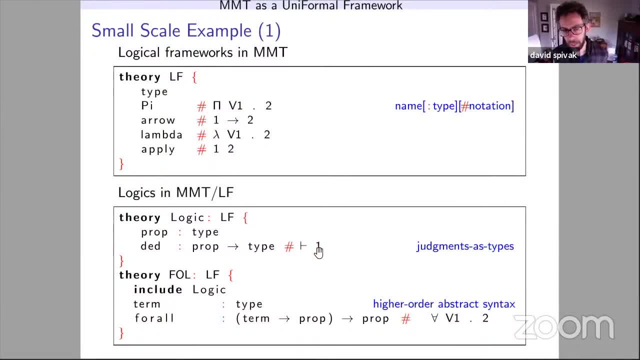 So in ded down below that one, does that refer to any other ones, or is it just? It's the first argument, meaning this one? Ah, okay, This is copied from the previous slide, so it's just first-order logic, as before. 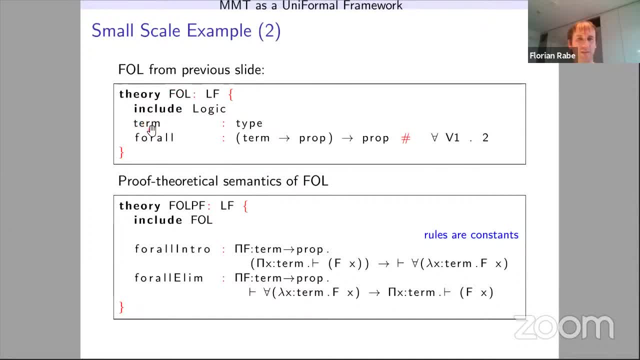 We have so far only declared the syntax. Now we're extending that with proof rules. We have default introduction rule and default elimination rule here as examples. All of this is relatively standard if you already know LF. If you don't know LF, then what follows? 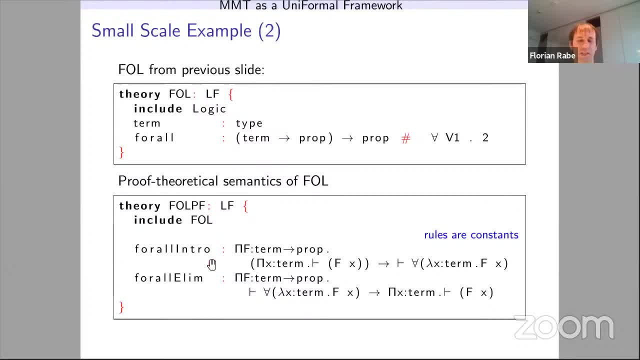 is a mini tutorial For representing logics in LF. So the introduction rule for first-order logic is meant to tell us how we can obtain a proof of for all x, f of x, where f is an arbitrary predicate on terms, And we do that by proving for every x. 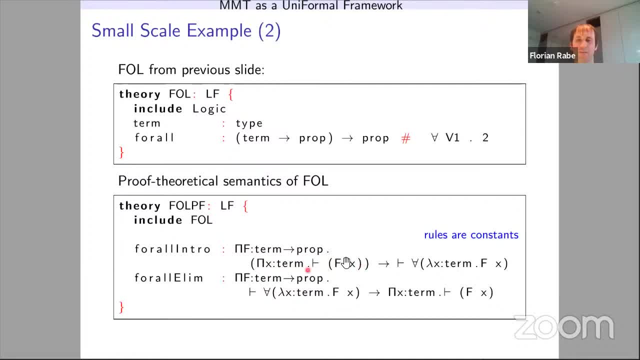 but f of x. So if we have a function that takes an arbitrary x and returns a proof of f of x, then that justifies concluding that we have proofed for all x, f of x. It's the standard Cari-Hart representation of proofs as terms. 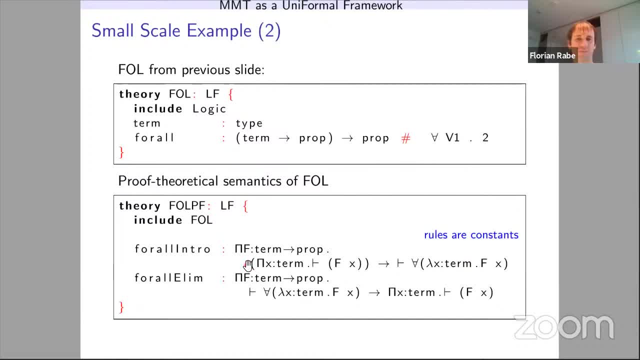 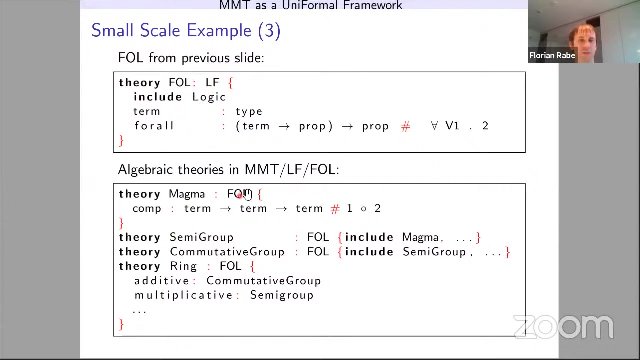 And the elimination rule proceeds accordingly. So that's the second level. After defining the logical framework, we can use that to define individual logics in it, And this is just a tiny example to showcase the modularity. Again, this is copied from before. Now for the third level, using first-order logic as a meta. 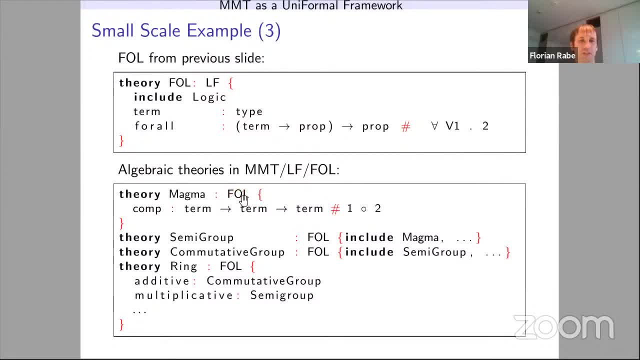 theory. we can now start formalizing some domain knowledge. In this example it's the algebraic hierarchy. We start with the theory of magmas, where we have a binary operation on the terms, the composition operation with its infix notation circle. 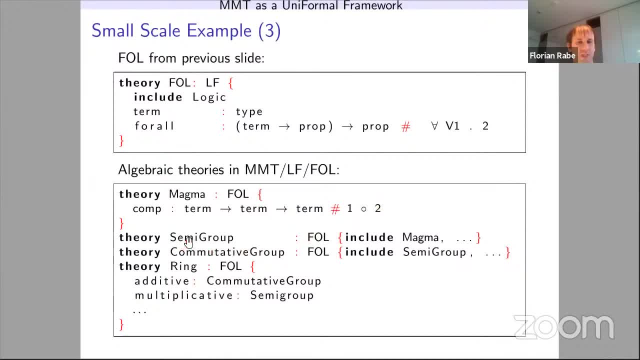 And then we extend that in various ways, for example to get the theory of semigroups, theories of commutative groups. And then one new thing we need if we want to do something like a theory of rings, where we need two binary operations. We cannot simply just include commutative group and semigroup. 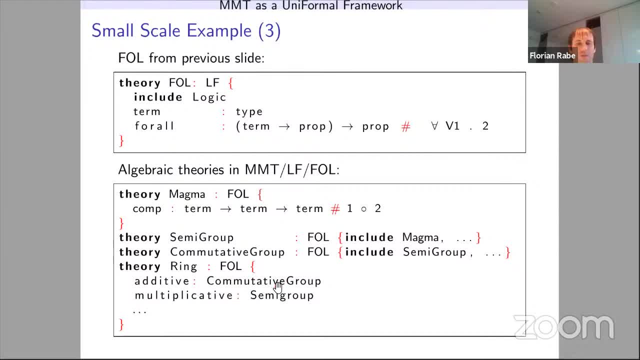 because they're supposed to share the universe of terms but they're supposed to be different binary operations. So we need a feature like named includes, to compute a copy of commutative group and a copy of semigroup, which we might call the additive and the marginal. 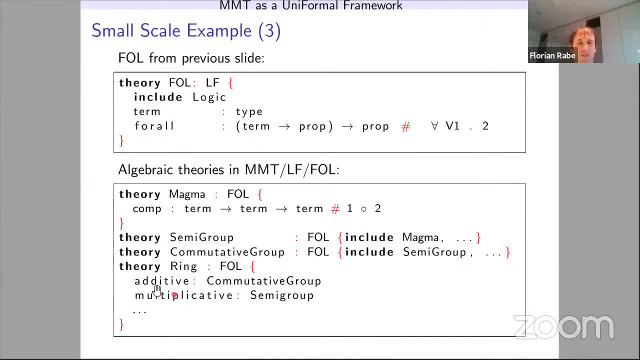 The multiplicative parts of the ring. And then we can do things like additive slash comp to refer to the additive operation of the ring and multiplicative slash comp to refer to the multiplicative operation of the ring. And of course, in practice you would add better notations for these operations, which I've omitted in this example. 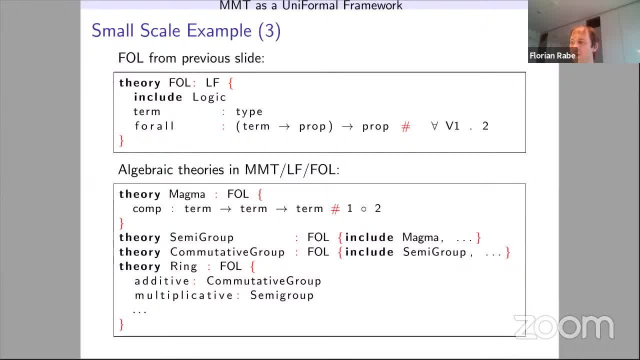 So that exemplifies the very simplest level how to use MMT. I'm seeing that people are asking questions in the chat. I had not noticed that before. Let me just check. Does MMT have a library of mathematics like Isabel or Lean or Misa? 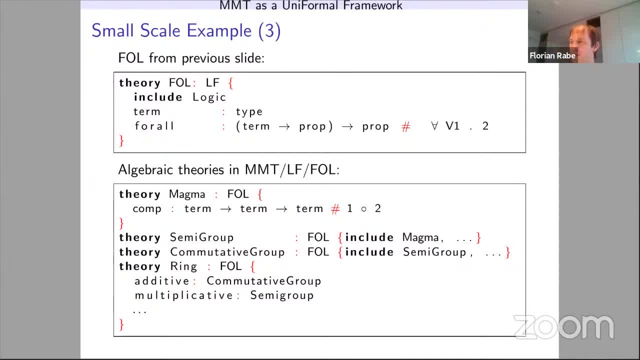 Yes, But again, MMT doesn't aim at competing with them in particular. Yes, But the way we think about MMT is that MMT doesn't have a huge library of proofed theorems because MMT doesn't have the kind of theorem proving support that Isabel Lean and Misa have. 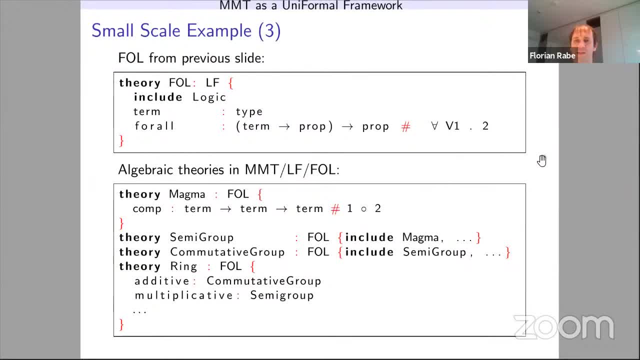 We have actually imported those libraries into MMT. That's something that comes on a later slide, So we can get back to that: The Big native libraries that are handwritten in MMT. that actually focuses on representing different logics, not so much different. 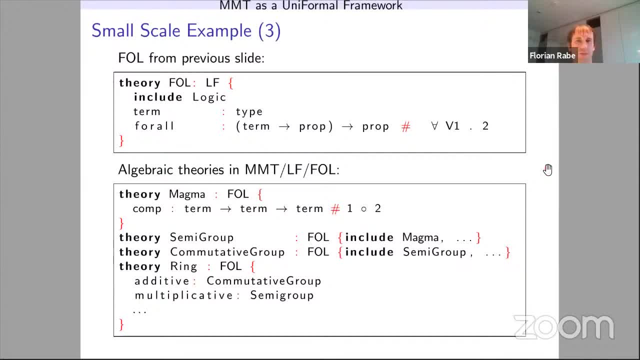 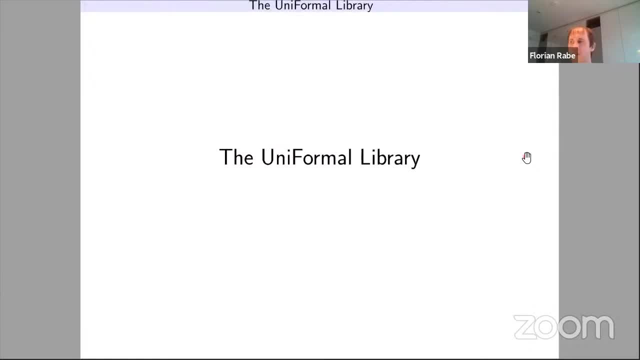 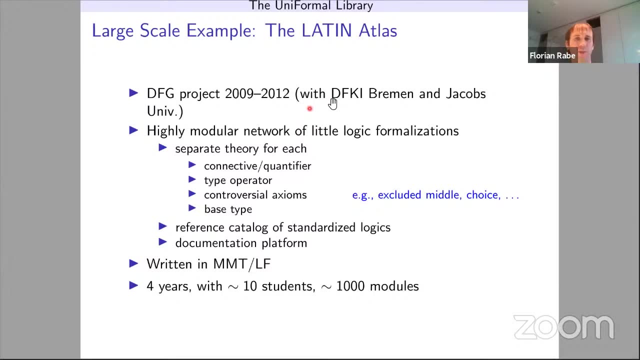 not so much large libraries of domain knowledge, And that's what I'm going to come to immediately next. So this is like the library of MMT. The MMT library started with what we call the Latin project. that was a collaboration with Tim Ozarkovsky from Raymond. 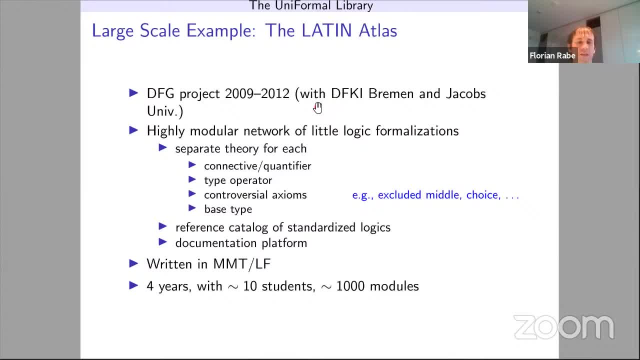 who maybe some of you know. And then the goal was to formalize all logics that exist in a highly modular MMT network of theories. So this was quite successful. It was the first major case study undertaken in MMT. Eventually we had one huge diagram. 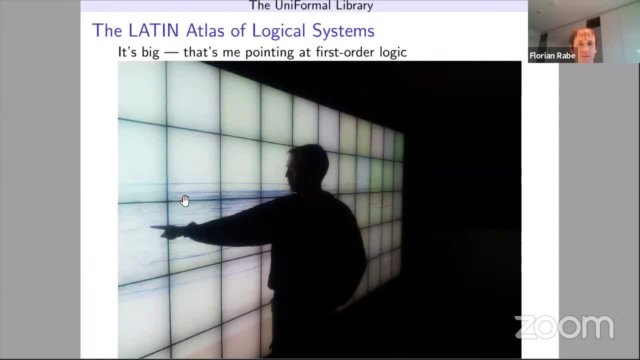 in the category of MMT. The diagram became so huge that we actually couldn't display it anymore properly. So at some point we visited colleagues in Paris who had a three by 10 meter screen array And for the first time we were able to actually show the entire diagram. 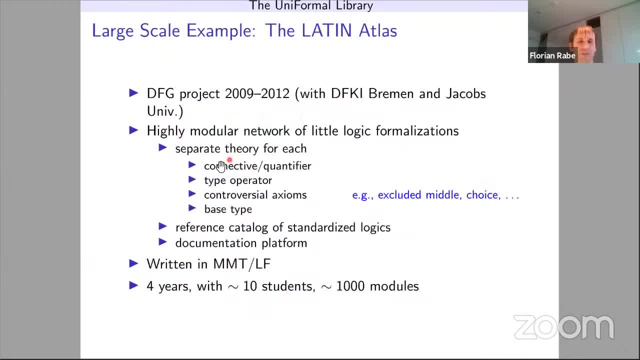 It gets so huge because of the principle that we state every single logical feature like conjunction or universal quantification in the smallest possible context means everything gets its own theory. X seems like excluded, middle or choice. They're all segregated into separate theories so that we can then build the logics that we need. 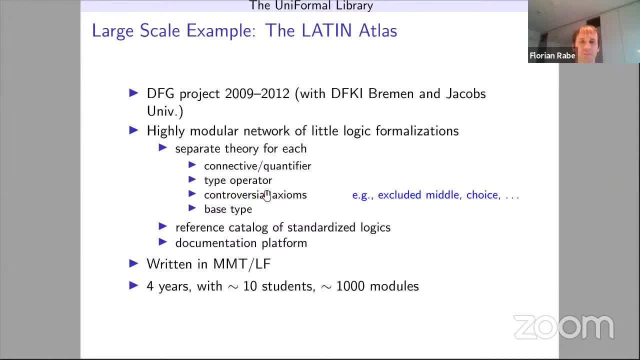 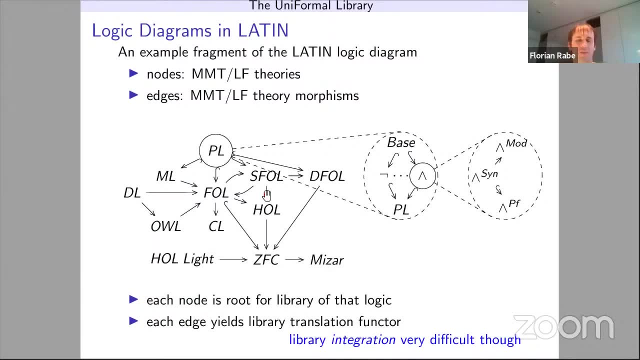 by importing exactly the features that the logic has. So we got the huge diagram. that was very difficult to work with here But didactic reasons is tiny fragment of that diagram. So we might start with propositional logic extended to first-order logic but also to sorted first-order logic. 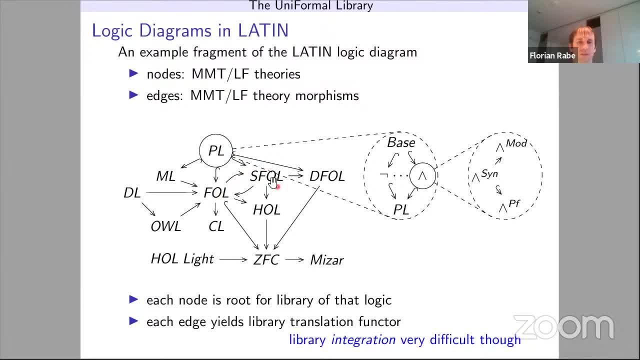 Then we have translations back and forth between those two. Sorted first-order logic then is the basis to build higher-order logic, where we basically have to add the function type operator to sorted first-order logic. Higher-order logic then has a semantics where we interpret types as sets. 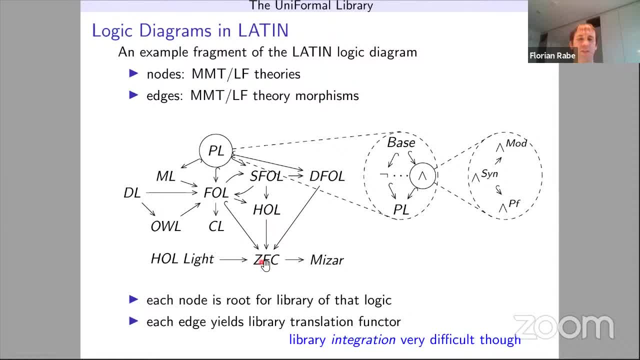 that we can write, as a morphism between MMT theories, into the set of C theory. So the C itself is formalized by extending first-order logic and adding the usual axioms of set theory. So you see, at that point the diagram does not commute. 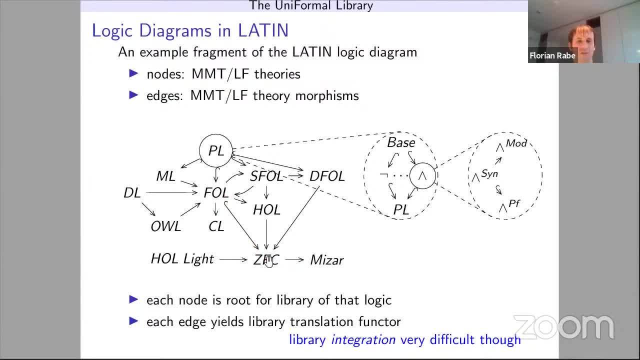 First-order logic is both the basis to formalize set of C and a particular logic that gets interpreted in set of C, And we can at this point start adding the actual logics of standard proof assistant into the diagram. Something like whole light is closely related to whole. 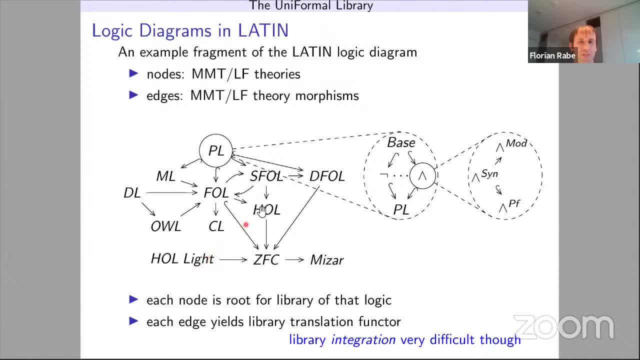 The arrows are not here yet, But you can imagine second inclusion error from whole to whole light, which then gets translated into set of C, And set of C itself is slightly weaker than the set zero of MISA. So we have another translation from there to MISA. 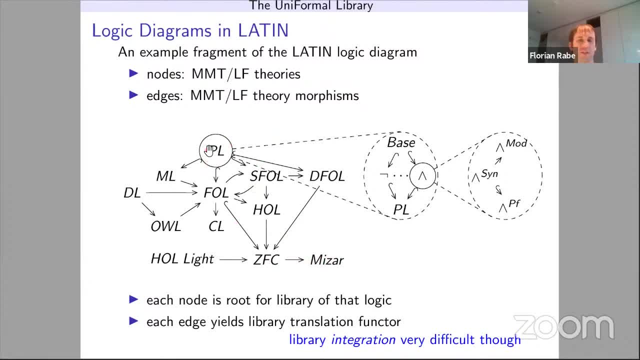 But that's just the high-level view If you zoom in. prepositional logic isn't actually just one Theory in MMT is written modularly, with all the features like negation and conjunction formalized individually and then imported as needed to form the prepositional logic we want. 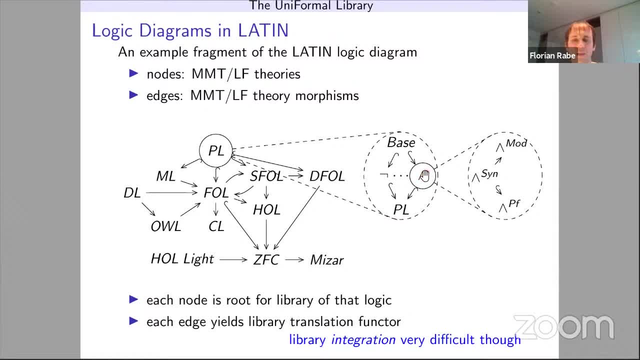 And then something like conjunction itself is not the single theory either. It's a triple of theories: one for the syntax, one for the proof theory and one for the model theory. And that's the special case where you only formalized one proof theory. 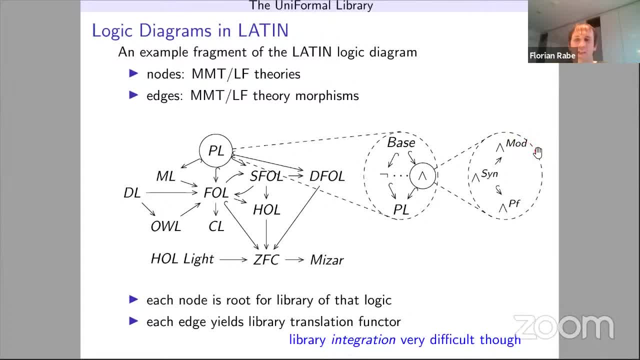 and then in the second case you just add one theory And then in the third case you only formalize one proof theory and one for the model theory theory. If you have a natural reduction calculus and a tableau calculus and so on, then you 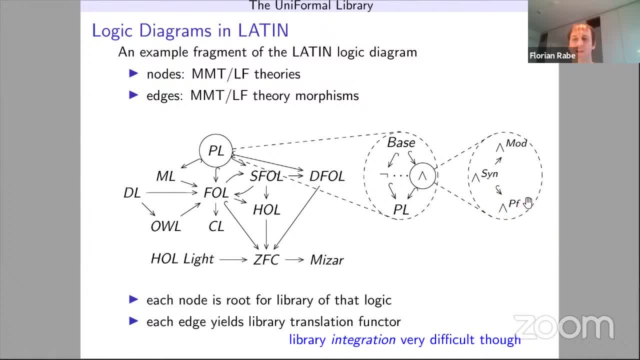 will actually end up with multiple proof theories here, and you can then represent meta-serums that relate those proof roots to each other as morphisms between the different formalizations of the proof calculus In the hierarchy of different languages. this whole diagram sits at the logic level. 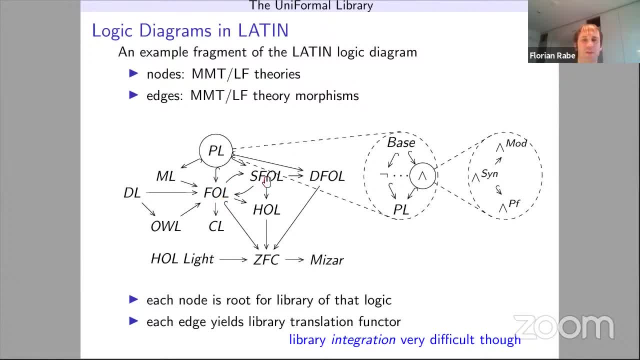 and every node in this diagram serves as the root of a domain knowledge diagram. So, for example, the library of MISA then is one huge diagram of theories, all using MISA as the meta theory. So in every node in this diagram you can think of 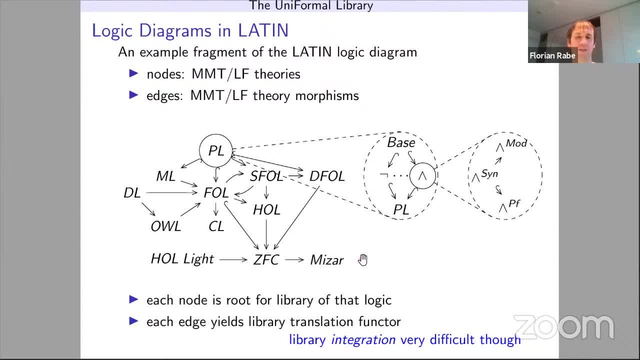 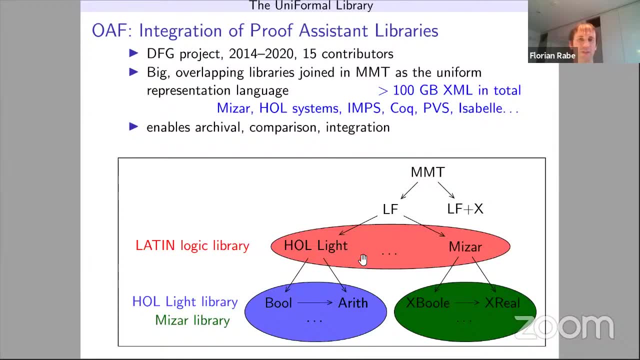 huge library dangling underneath it for the concrete domain knowledge written in that logic. That brings me to the second major project we did. That was the OAF project. OAF stands for Open Archive of Formalizations, And there we attacked the problem of integrating all the big proof assistants into this diagram. 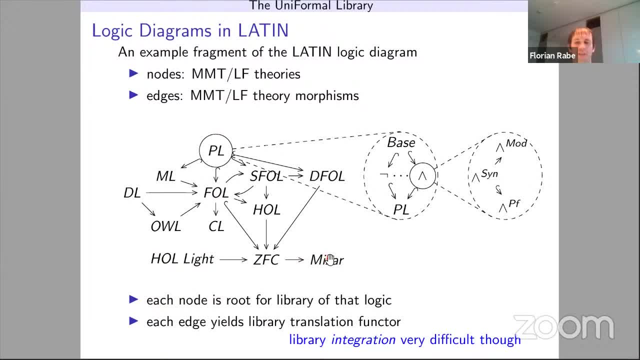 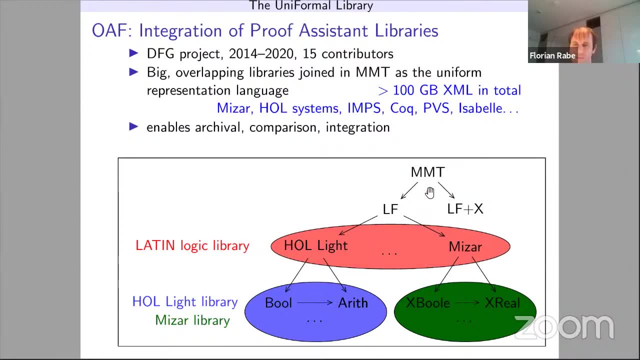 So already indicated here that we have proof assistants in the diagram And we can now take those logics, treat them at the base of a logic And then we can generate the library like the entire whole library or the entire MISA library. So when we speak of library development in MMT we have to distinguish between: 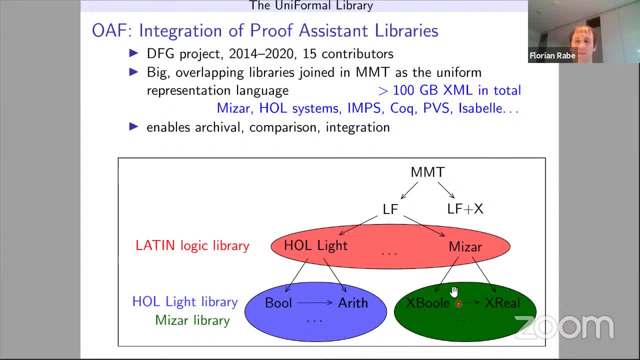 the manually written libraries and the generated libraries. This level is usually where the manual work sits, And then we have huge libraries from concrete proof assistance that we translate into MMT. When we translate into MMT we don't target MMT's concrete syntax. 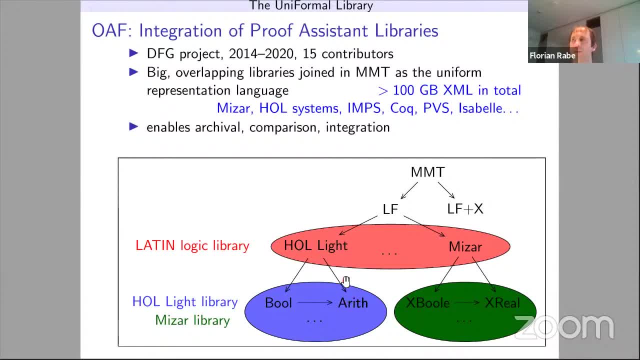 We target its XML syntax, which is based on CodeHouse's Omdoc format. But recently, especially when we did the Isabelle and Coq libraries, XML became actually not scalable anymore. The individual files just became too big. So now we're working with zipped XML actually, because otherwise we have to stream all the 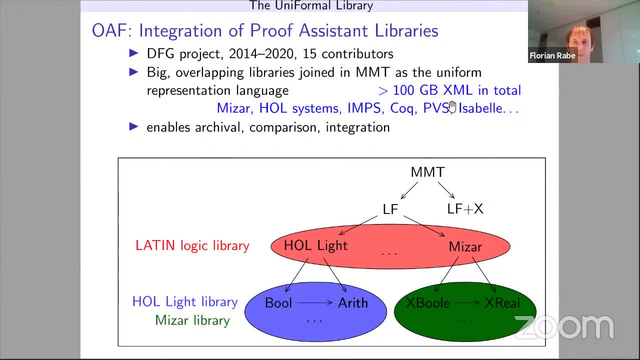 files through compression software, because otherwise the files on disk grow to gigabyte ranges where we just can't work with them efficiently anymore. But with that we were able to take the libraries from six major proof assistants and translate them all into MMT-compatible XML. 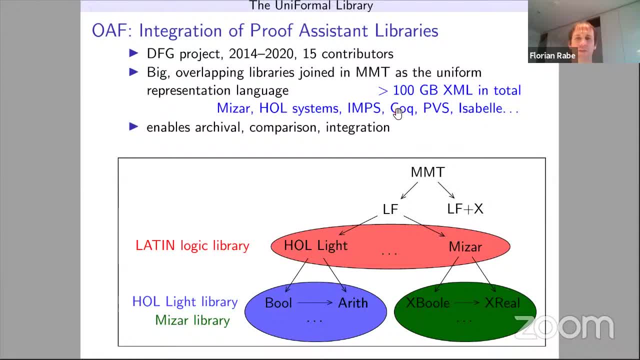 That was a huge undertaking. The problem is usually that it's extremely, extremely difficult just to write one of these importers. We always focused on completeness, actually covering the entirety of the language, And that's really hard because every one of these proof assistants has numerous you. 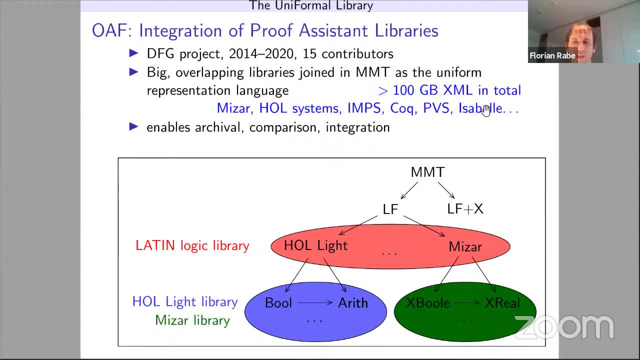 name. it features arcane idiosyncrasies, experimental features, legacy features that should be abolished but can't because you people have gotten used to them, which make it really hard to represent them in logical frameworks. So basically for whole we can still kind of do it in LF, although already there. the 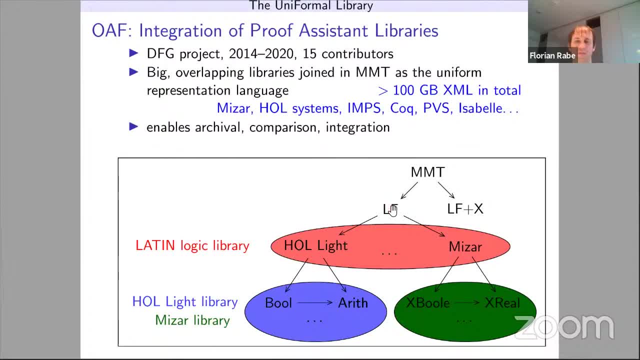 type definition principles. So lots of whole don't really work nicely with LF anymore. So basically, all the time we have to come up with new logical frameworks. That's what the plus x here represents: Coming up with appropriate frameworks good enough to adequately capture the logics. actually, 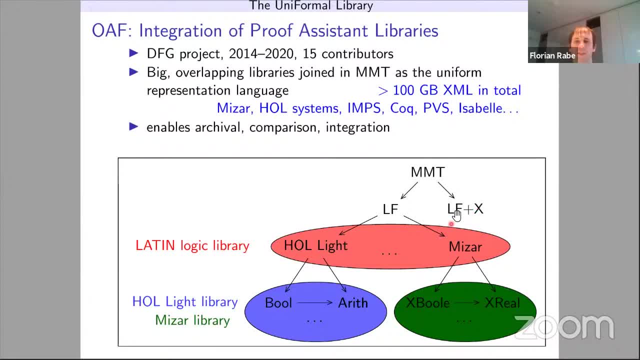 used in practice. And that's then where MMT shines, Because usually the x that you need is a surprise. So you dig into one particular system, like, say, PVS, and you spend a month implementing and communicating back and forth with the PVS developers to truly understand what the 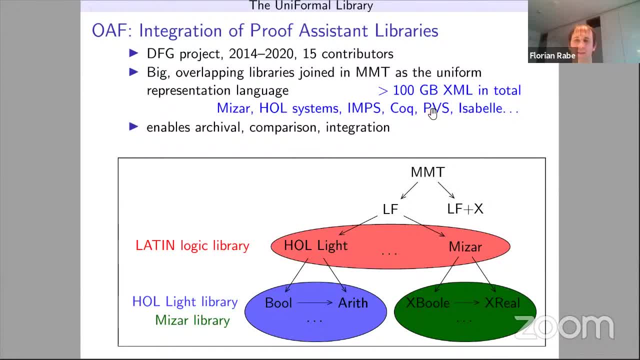 various subtleties in PVS actually mean- And halfway through you realize- major complications at the lowest levels. Okay, So we have to come up with the appropriate framework feature to actually represent them. That's why, even though we worked on this for six years with quite some funding, we 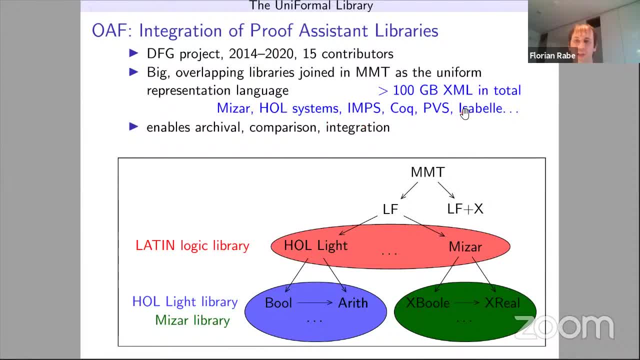 were only able to import these systems into MMT, We have not really been able to do much work towards integrating them with each other. So now we have, say, the Booleans of whole light In MMT, but we also have the Booleans of MISA, and those are currently side-by-side without 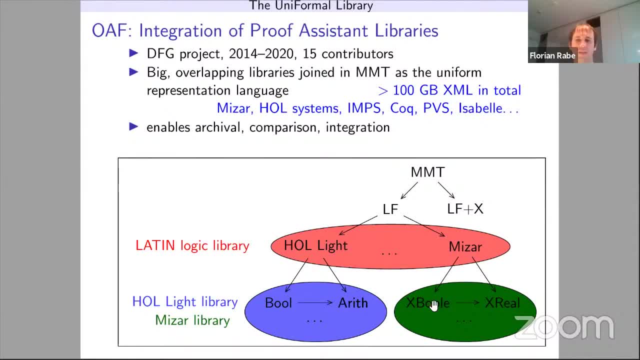 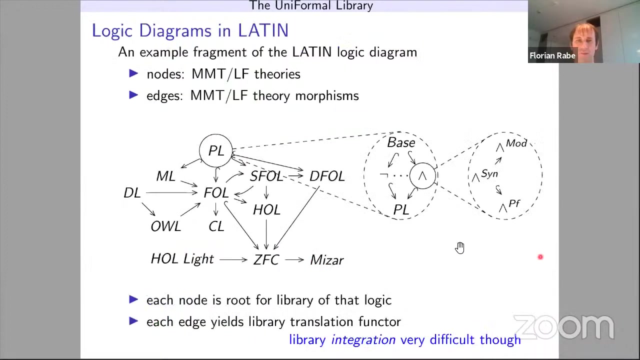 any relation between them. We've done a couple of initial experiments on figuring out how we can integrate these concepts across libraries, but that remains a huge problem. Okay, Next slide. please Question in the chat In the previous slide: are functors in the diagram category the functors or not? 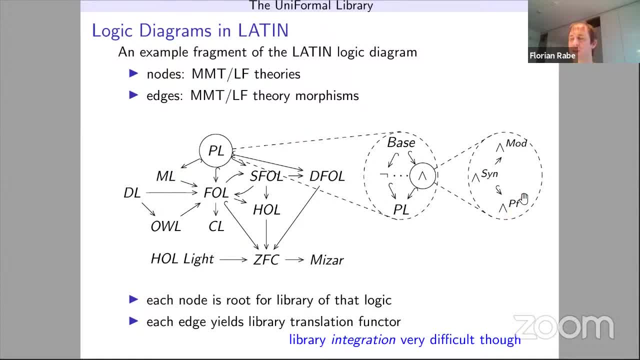 So this is a diagram in the category of MMT theories and theory morphisms. So every arrow here is a morphism in MMT. I can go into details of how these morphisms work, if there's interest. Additionally, you can think of every node in the diagram as a morphism. 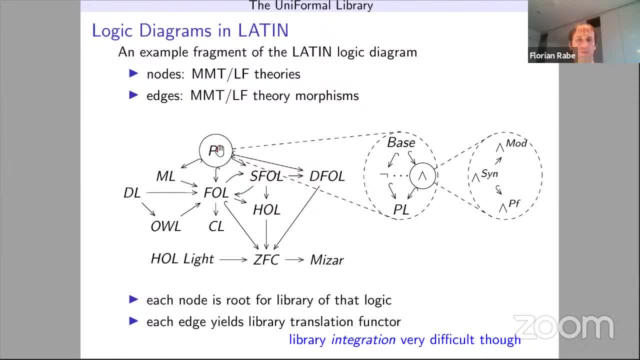 Okay, And this diagram is inducing a category, formally as a slice category, namely all MMT theories that extend, for example, first-order logic. So any content formalized in first-order logic becomes an MMT theory that extends first-order logic. 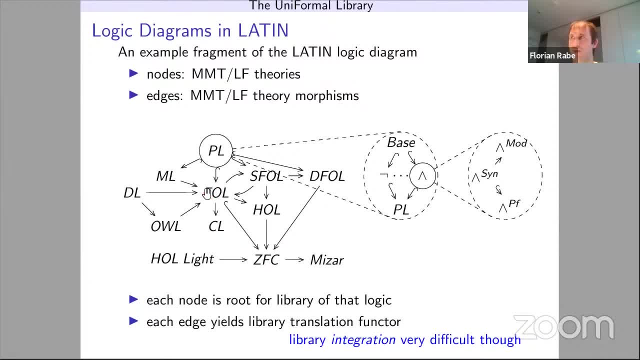 So you have the slice category under four And then, via push-out, every one of these arrows can be seen as a functor between the slice categories. So you can think of them as functors that translate the category of four theories to the category of S4 theories. 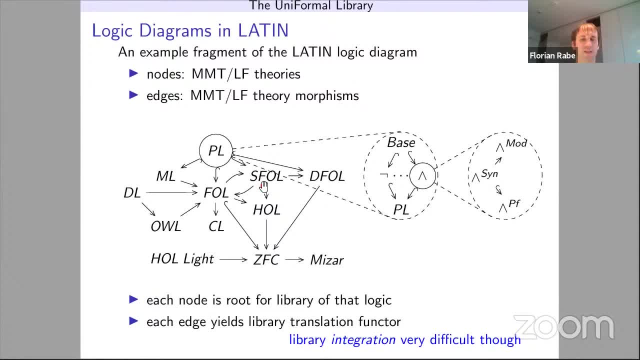 So much for the theory. In practice, it turns out, push-out works only in a few cases as an adequate primitive for presenting translations between logics. Current research is going beyond that, figuring out how we can still maintain nice, categorical intuitions but also being able to represent much more complicated translations than compositional. 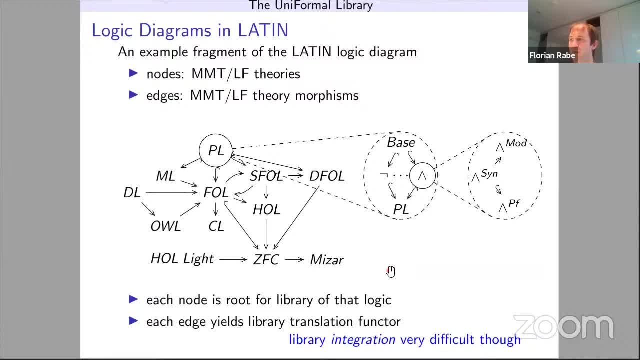 ones. Yeah, so generally, MMT formally doesn't distinguish between- oh sorry, I'm answering the question in the chat on whether there's a difference between logical frameworks and logics in MMT. So generally, MMT logical frameworks are just theories, like any other theory. 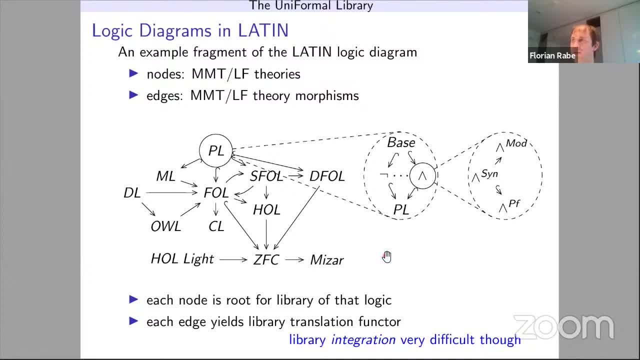 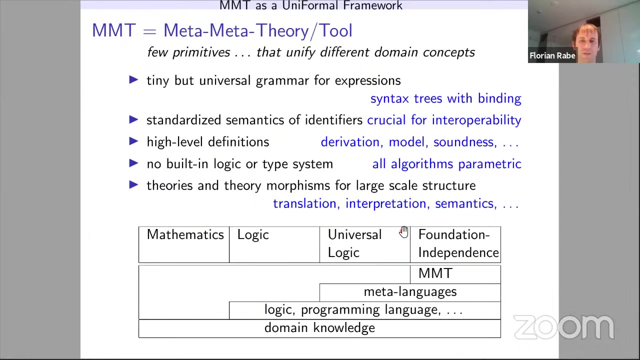 So there is no conceptual distinction, There's only the meta-theory relation. There's no definition where one MMT theory can designate another one as its meta-theory. So the distinction between the four levels here is entirely pragmatic in how you use MMT. 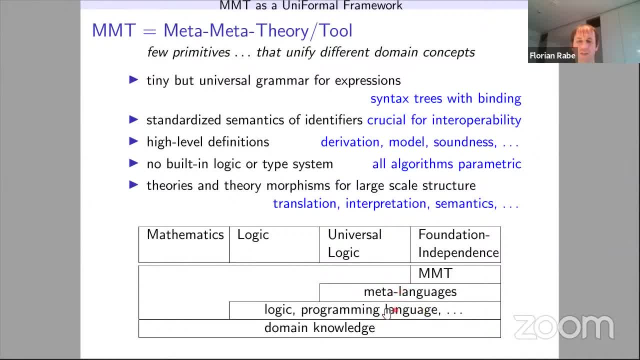 So these are languages that occur as a meta-theory of these And these occur as a meta-theory of these. Now, there's one difference, so to speak. Usually here you need to inject some rules to get off the ground, to get the semantics. 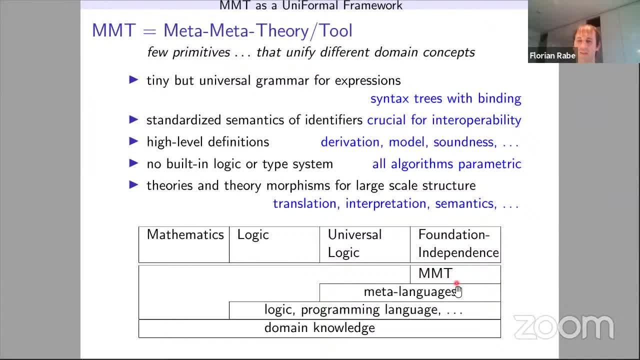 of the frameworks, And then usually you don't need to add rules anymore down here. I think that's why in the paper that is referenced here, there's a bit of a difference in the definitions, Because I needed to account for the fact that here it's not enough to just divide. 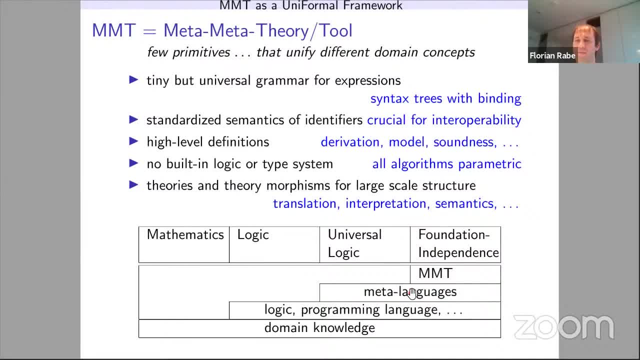 an MMT theory, You have to inject some rules as well. But actually in MMT you can inject rules at every level. It's just in practice. usually you only need them here. Ideally you only need those extra rules here. 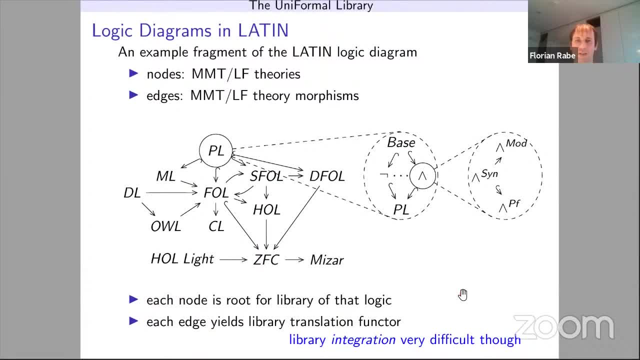 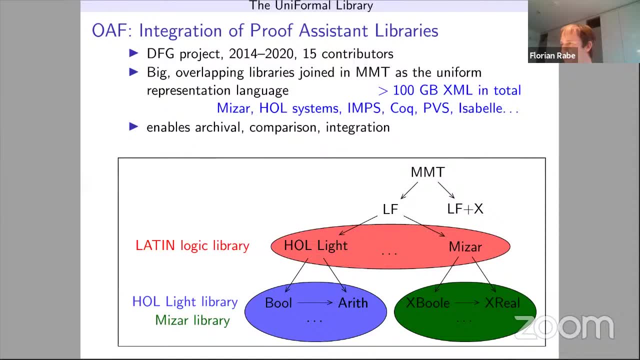 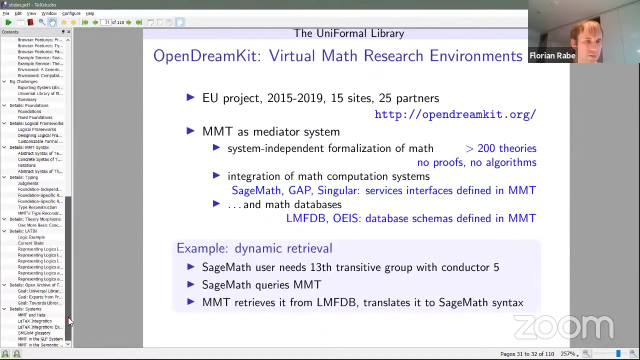 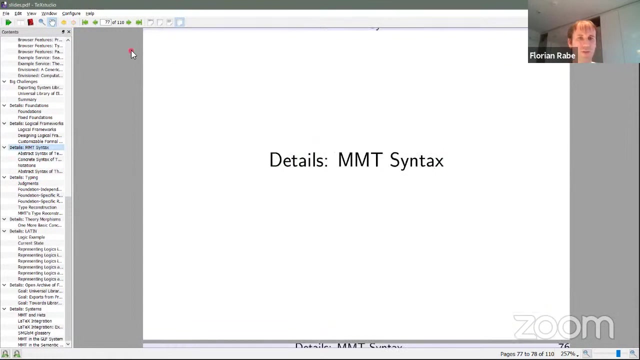 I can go into details regarding the kinds of rules that are needed. I can also go into details on the definition of theorymorphisms. Okay, let's do that. Let me briefly do a little bit about the syntax as well. That would probably be helpful. 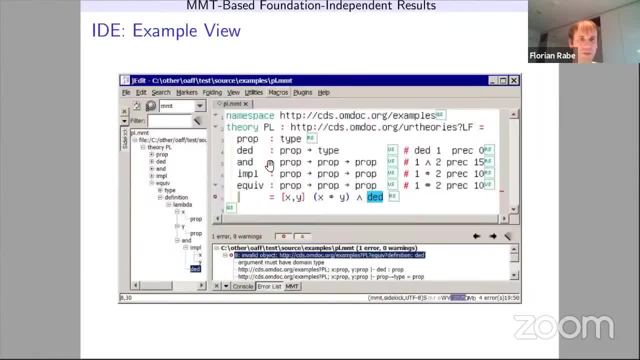 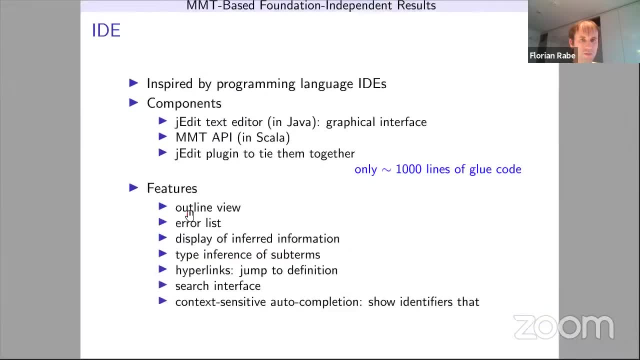 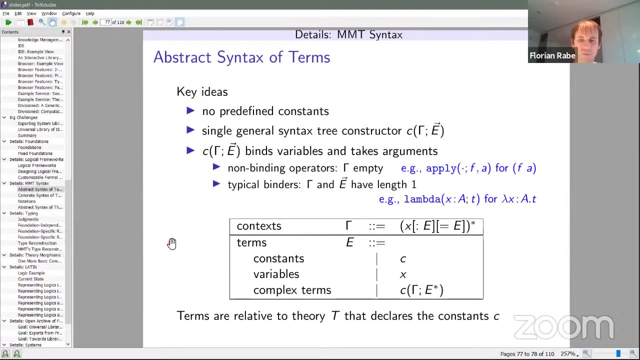 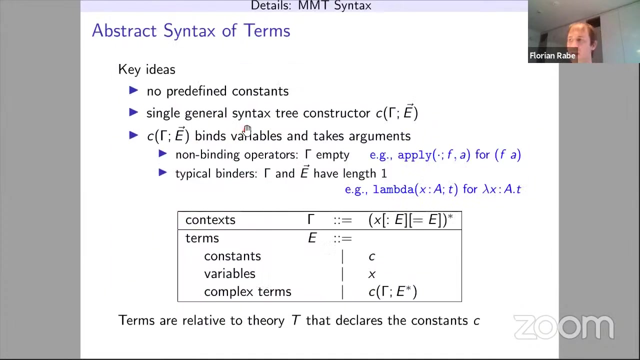 The lady has the keyboard over here. It's not sure if I'm being corrected… Okay, So since people hi the chat asked about the details of theorymorphisms as well, I'm gonna do that again in a second. Okay, Now, if there's some showing about it in three or four verses, just go to number'mi. 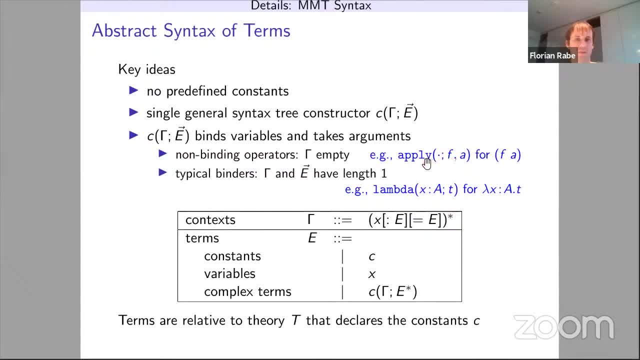 let me give a little bit of more formal details. In the simplest possible incarnation, this is the grammar of MMT. You have constants which are declared in the series, variables which are declared in context, and then complex terms which may bind some variables. 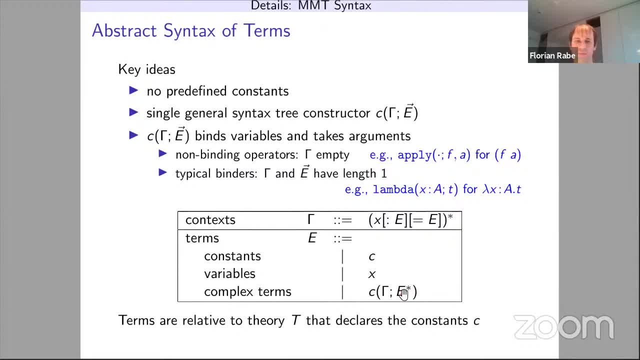 and which may take some other expressions as arguments. Then, for example, the concrete syntax like lambda x, colon, a, dot, t, which you have to want the user to write, in which the parser has to recognize internally, becomes something like the constant lambda. 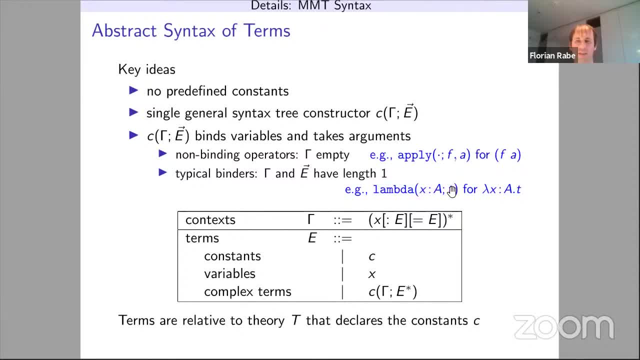 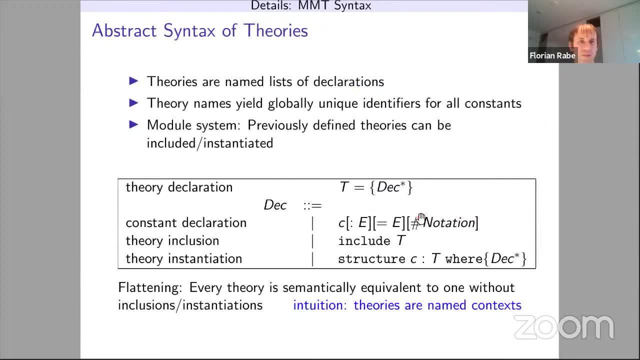 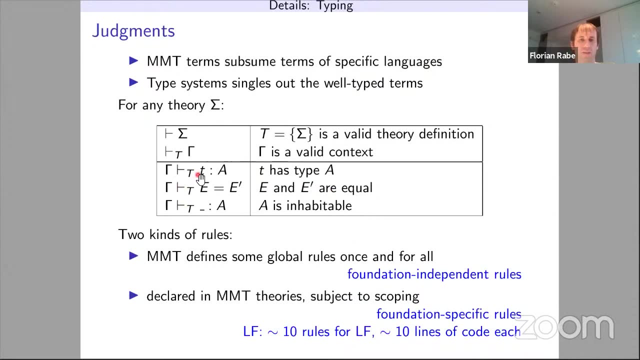 binding the variable x and a and taking t as a single argument. On top of that, MMT declares some judgments. First of all, there's a binary judgment between expressions for typing and another one for equality. Both of these are relative to a theory. 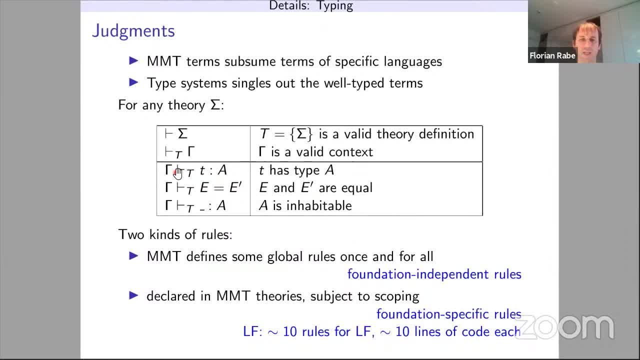 and the context of three variables, And there's a couple other judgments, but these two are really the essence. In the next lecture we'll understand how customize models can be applied, in which direction, and then show you how overall. Now, MMT defines all the system-independent typing roots. 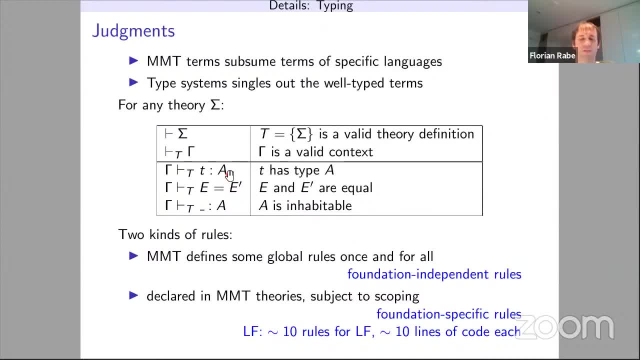 once and for all, and then every system can act some typing route of its own. For example, for LF we add lambda as a constant, so we have to add some typing roads for lambda, like type inference, equality checking and so on. 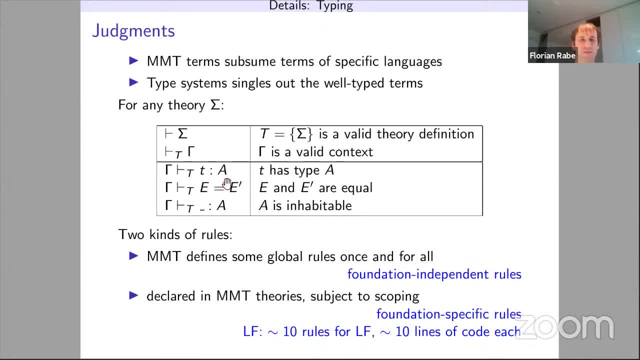 You just use LF to add unknown versions. these are provided as little code snippets, just a couple of lines, And then from that MMT generates the type checker for the respective languages. In the case of LF, we need about 10 roots. 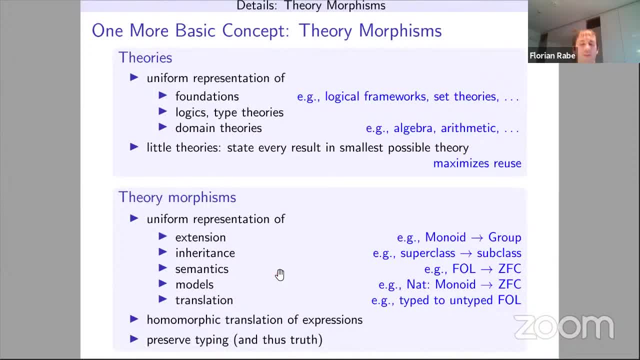 And then from there we can go to theory morphisms. The general idea is that the theory morphism uniformly represents compositional translations from one theory to another, So they are homomorphic translations from one language to another, meaning a theory morphism from. 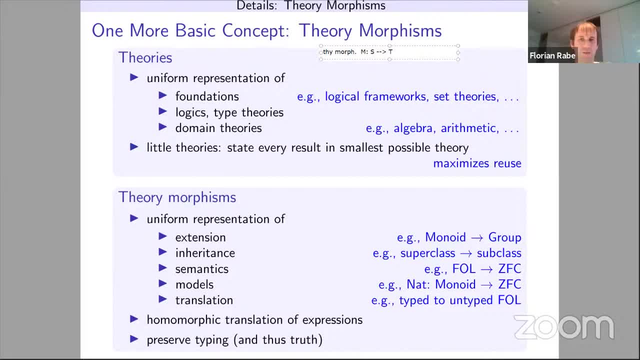 any two generations in this case, whether that's T the dominant or some other�ルreaming translation here. So a general idea about the theory morphism is that�� основan計, a neuromorphic translation, einmalik is the differences between safe removal of the 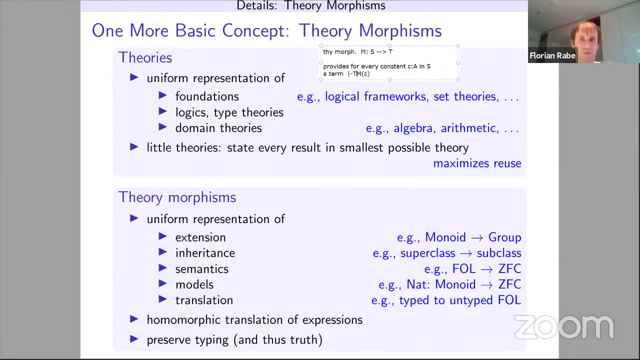 language and safe removal of a language in Dese 99.. When we take into account the notion that the type meetings of C, E, So the composition idea that limitedесто Correspondence to absolute Estáclass, tant the term M of C relative to the theory t, and now that must have type M of A, A Well, doesn't that make sense. 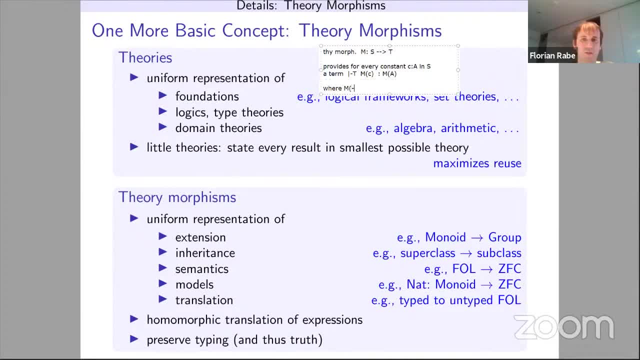 Well, we could do that, even if we wanted to use some value solution and say: Well, where M of is the homomorphic extension. So this is basically how morphisms are defined for most formal systems. For example, you find that in first-order logic. 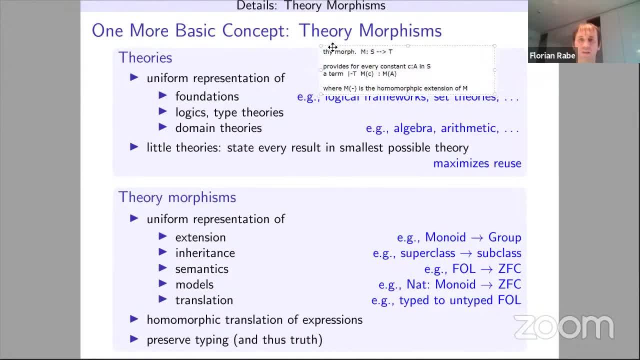 in exactly the same way. Institutions are what provided the inspiration of this kind of approaches. Except NMT realized that you can actually do that generically, once and for all. And then, once you fix the meta-theory like first-order logic and you've taken the appropriate slice category, 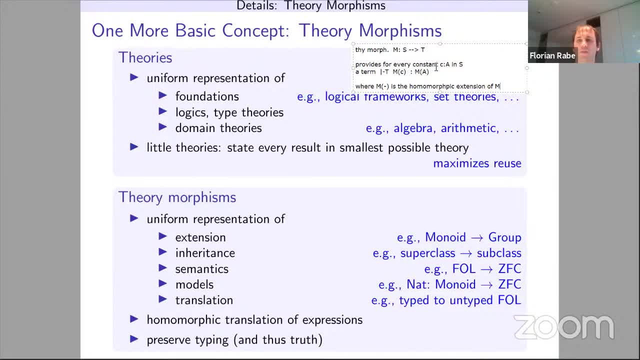 of theories extending first-order logic. you very nicely get the category of first-order logic theories and morphisms. So the main idea is we have one huge category of all theories you might want to write down ever, and then morphisms between them And then when you define concrete languages. 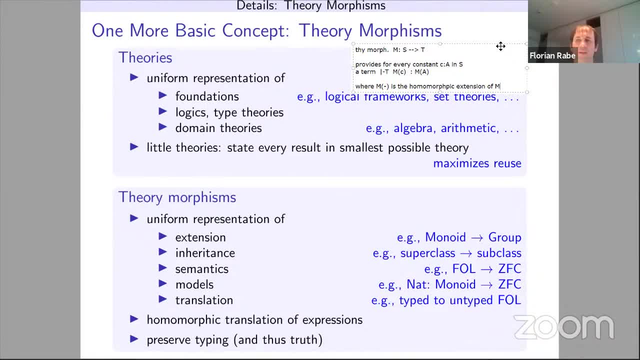 all you have to do is single out the appropriate subcategory, It turns out. we can then use that at all levels. We can represent, for example, modular development of logical frameworks in the same way as translations between logics or as morphisms between algebraic theories. 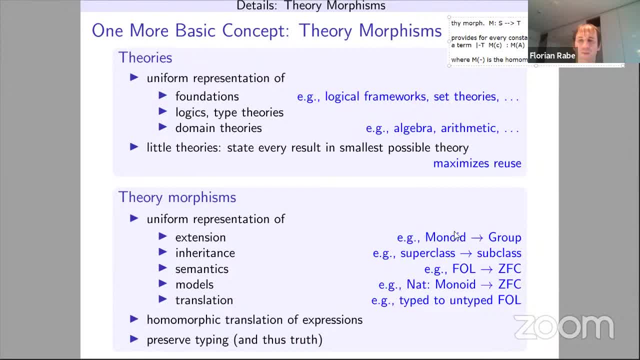 So, for example, the fact that group extends monoid by just adding the inverse operation and its axioms is a theory more or less than NMT inherited, but it's a theory more or less than NMT inherited, but it's a theory more or less than NMT inherited. 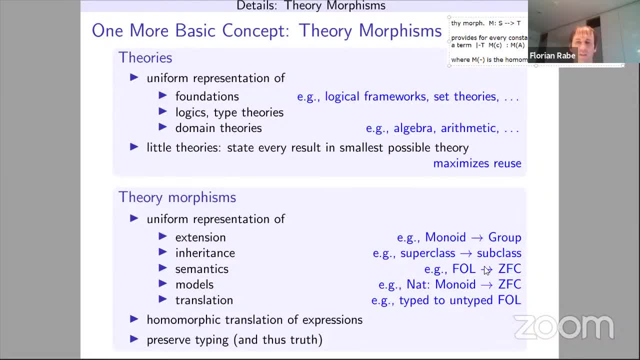 but it's a theory more or less than Yเป, but it's a theory more or less than Y보ğ, but you幾 chance that it actually comes from E gems' And in many cases there are juezown's that are based on rape. 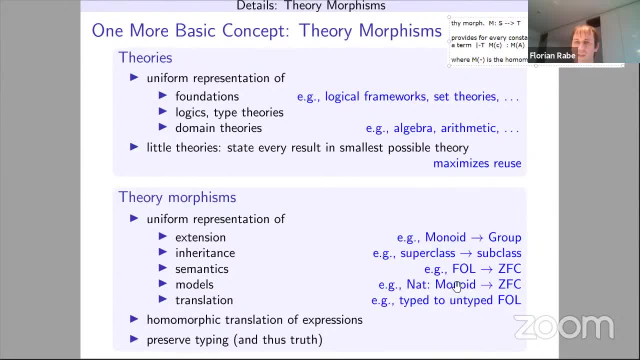 from the theory into your fixed background theory in which you formulate your semantics. So this could be a particular set theory, a particular programming language could be a particular proof assistant, depending on what you use as your ground truth to get off the ground. 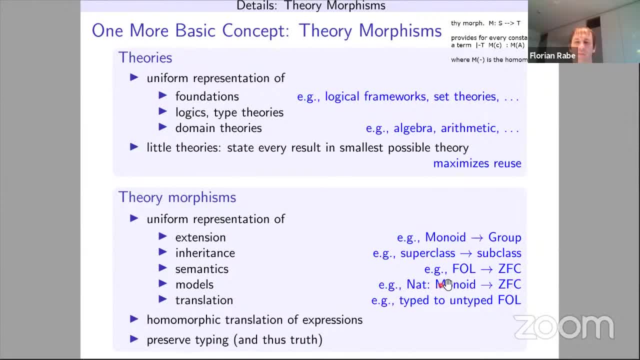 Models are then just morphisms from the abstract theory into that theory And lots and lots of logic translations, like negative translation, from intuitionistic to classical logic, the other way around, classical to intuitionistic- can be represented as theory morphisms in that style. 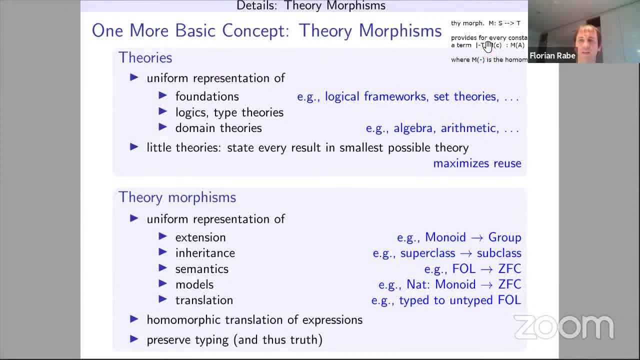 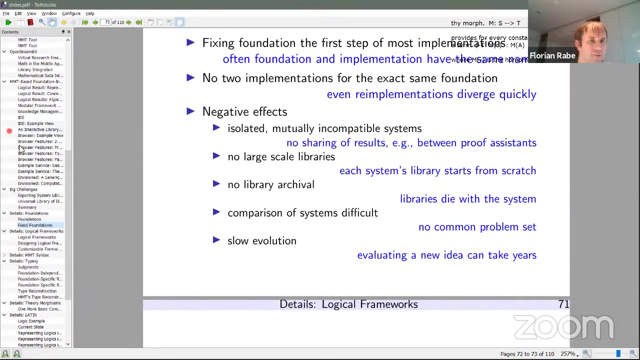 And it all goes back To the key property that morphisms must preserve all MMT judgments, in particular typing and equality. So let me circle back to some kind of conclusion. What's the most interesting? What's the most interesting to say next? 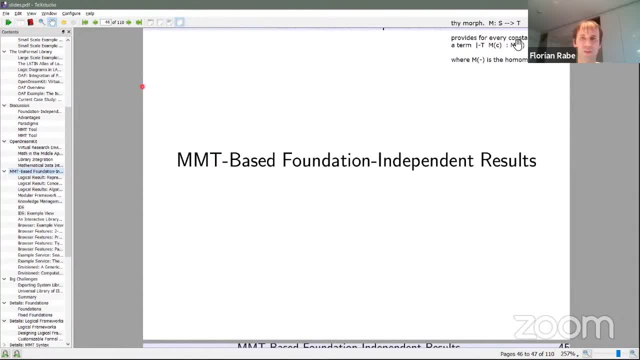 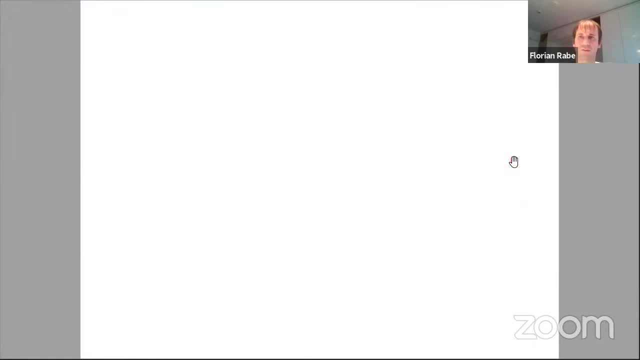 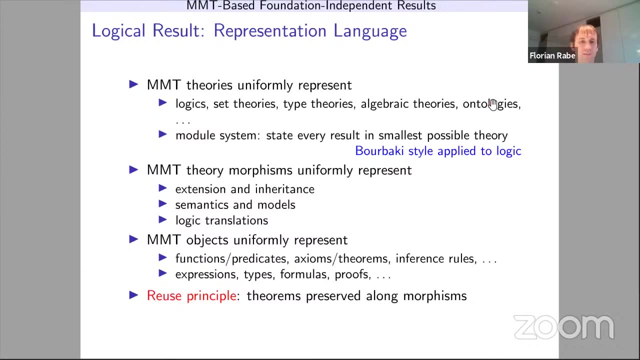 Maybe I briefly give you an overview of some results. So we've used MMT series as a uniform representation language. So we've used MMT series as a uniform representation language. I've shown you that. I've shown you that too, Algorithms implemented on top of that. 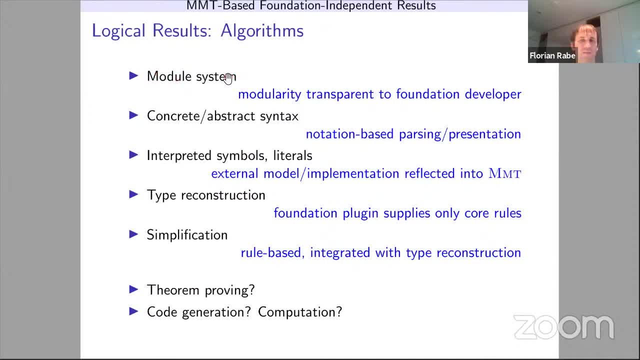 So I've indicated the module system, I've indicated that there is a parser for connecting concrete and abstract syntax and similarly a presenter to render everything either as text or HTML. I've not shown you, but I can tell you. now one of the most advanced results is a generic type reconstruction. 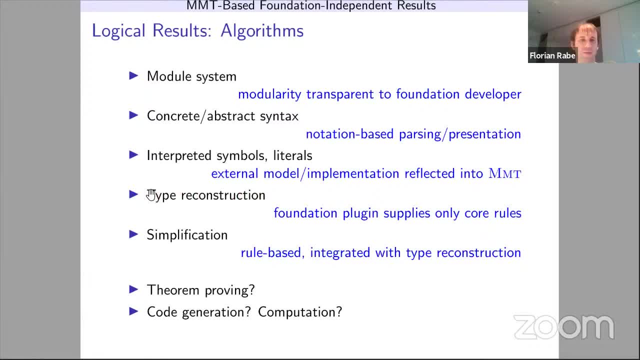 I've shown you that. I've shown you now, one of the most advanced results is a generic type reconstruction. I've shown you that. I've shown you that It's dashed from inaudible 007 007 to about 20% in 60 seconds. 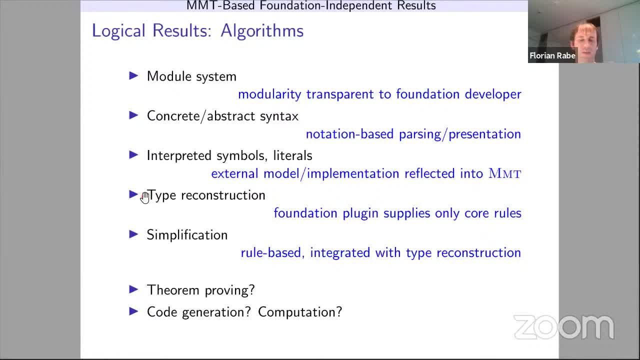 It's done. defense- 오늬同等 베 network, which is answered by dynamic, fundamental and negative, say death. So there were seeking for vibration instead of speak inおお 2ọ, 007, 007.. It's just an interactive system: whereivity. 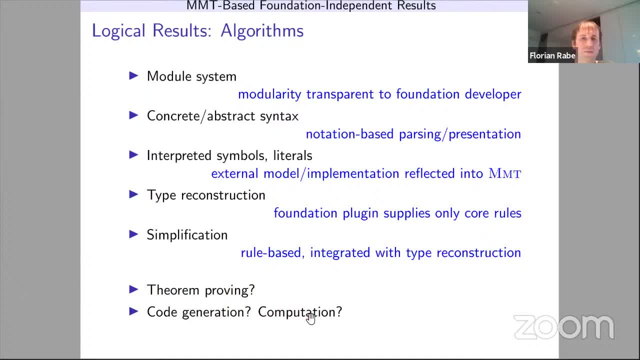 It's an interactive system with kinetics, the same function as clockwork, For example. You do some elements, It's more than a float. It ends with salv positives. Those are things where MMT can in principle also be used to take the existing techniques. 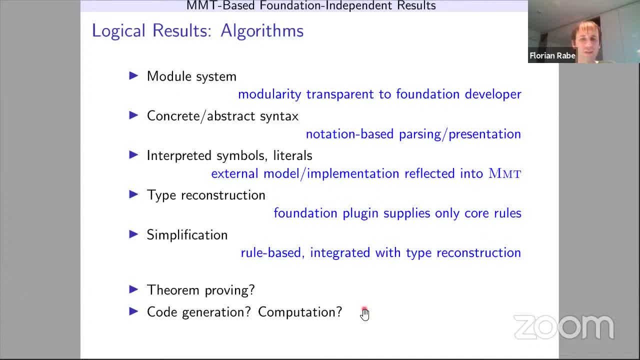 and generalize them to language-independent levels. It's just that it's hard to compete with the existing systems and it's hard to enable students to write papers about those things, so we've deprioritized them in the past, but that is something that we're working on. 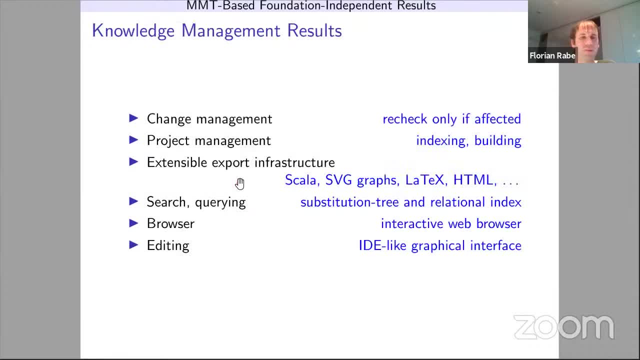 Those are the logical results. We have a lot of knowledge management results as well. That was the original motivation of MMT: that if you fix the old infrastructure for how languages are defined, you can then implement generic services that every language needs but that no one wants to implement. 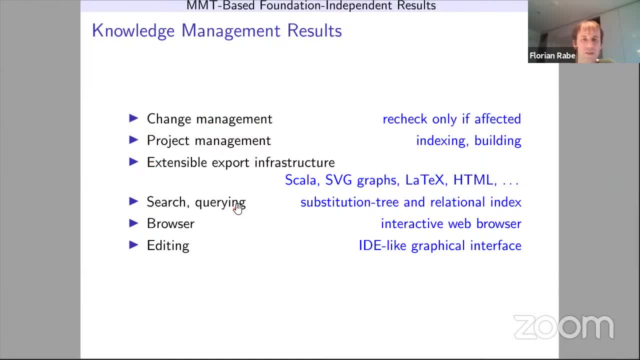 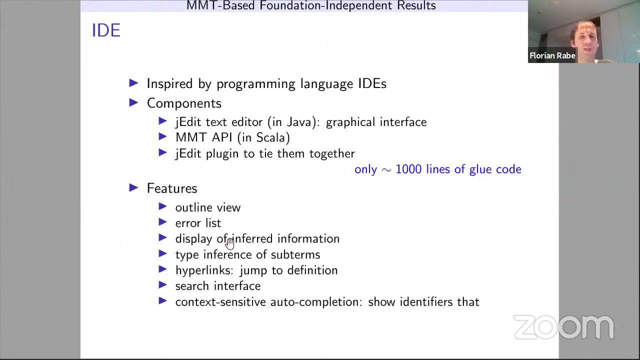 like change management, search engines, editing in the browser, all these kind of things which we can implement once and for all and often relatively easily in student projects, but which would be extremely difficult to build for any one particular system. Showing you a screenshot of the IDE: 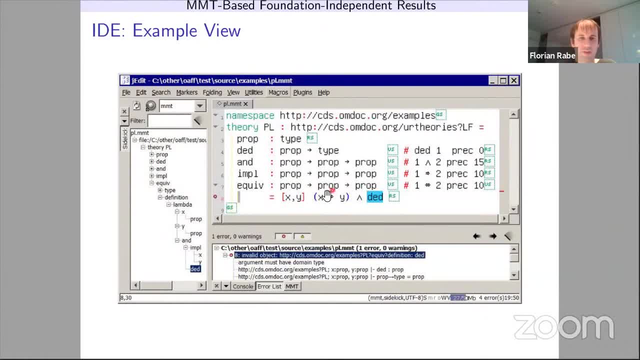 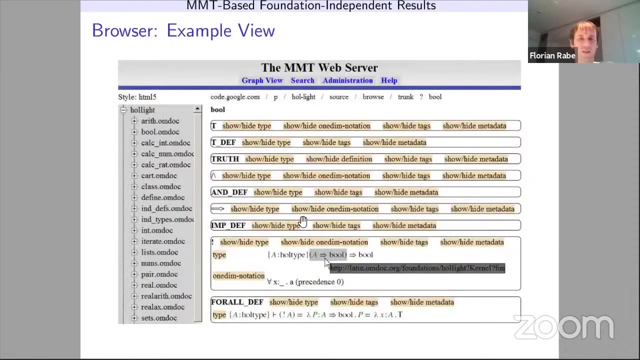 Here's an example of the type inference I mentioned earlier. For example, here accent1 are given as bound variables without type, and the system notices here that these are made a mistake. This is the HTML browser and this is the whole light library. So here we have the universal quantifier of whole light. 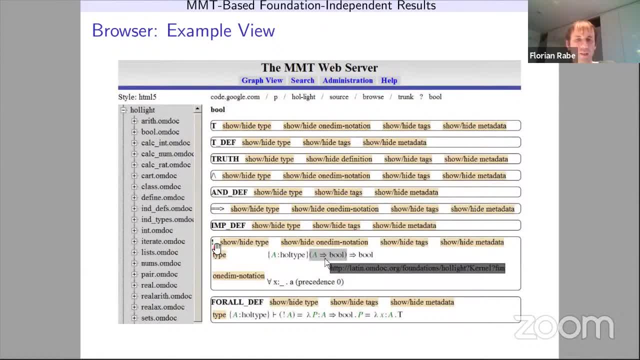 That's one of the libraries that were imported in the OAuth project. So for any whole light type we have, for any predicate on A, the universal quantifier that gives us the universally quantified formula. And now you can hover in the browser and MMT does the type inference. 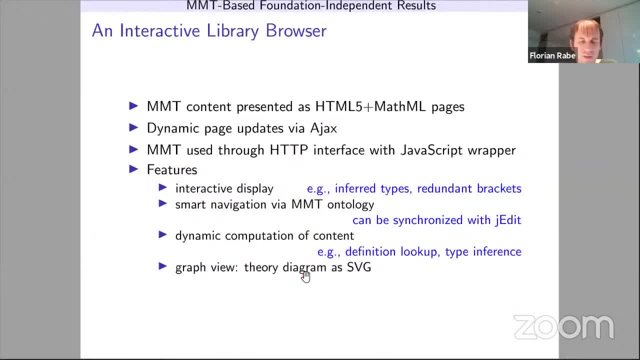 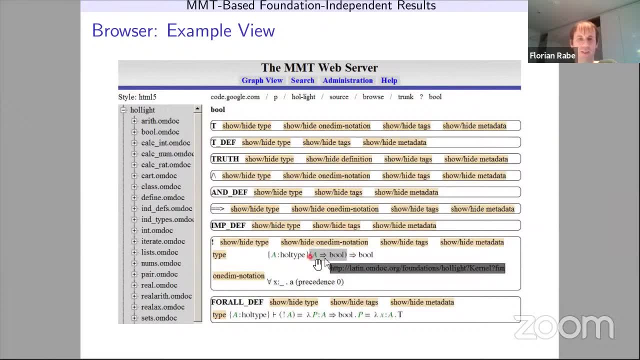 for that system. I saw there's a screenshot on that. It's not here, But anyway, so MMT should. after selecting a term, you can right-click on it and you get the type inference In the browser. that's a very difficult thing to do because 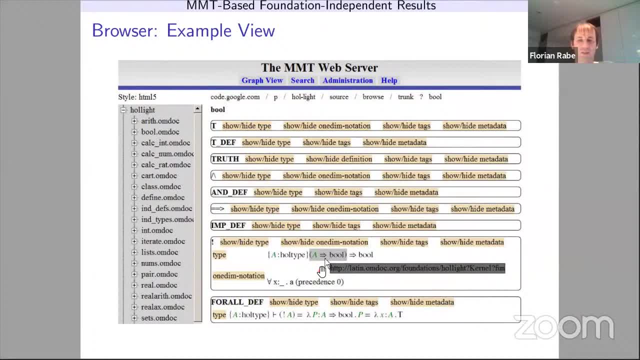 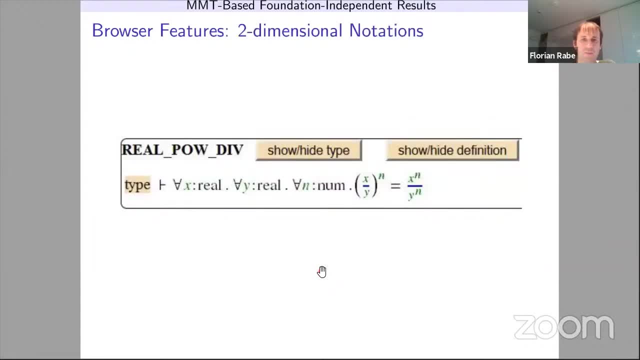 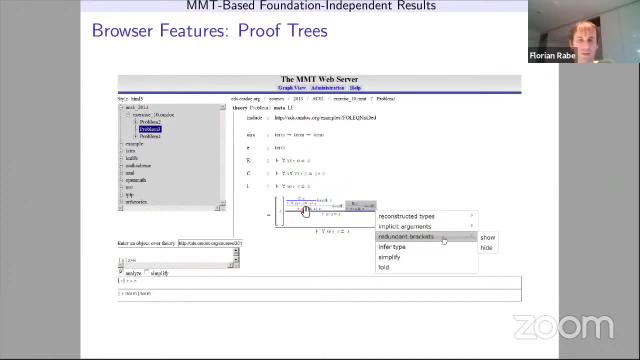 the browser has to be aware of the semantics of your logics, which, in the case of MMT, works, because you can just run MMT as a backend. Here's a very nice mini application that I did for my course. I just used a different set of. 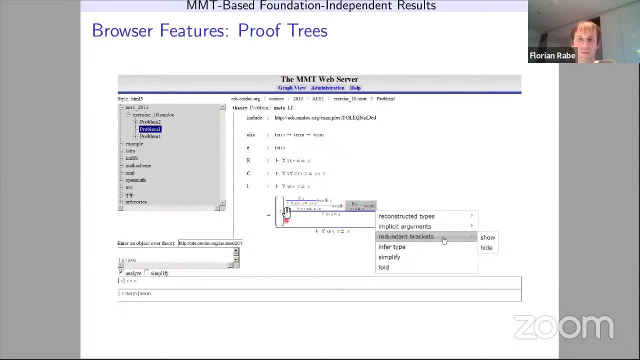 notations to get proofs rendered as proof trees, In particular all the intermediate formulas that are derived during the proof. they are all obtained through type inference. that happens dynamically in the browser when the proof is shown, And the cool thing about that is it works for an arbitrary logic as soon as you have the rules in. 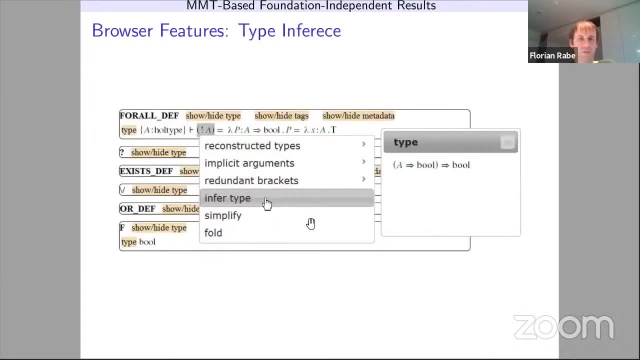 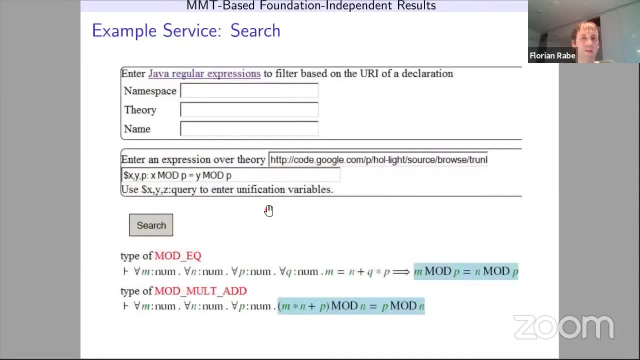 MMT. Ah, here's the screenshot for type inference that I mentioned earlier. Here's an example of generic search, again for whole light. You enter an expression with some free query variables- in this case x, y and p- And you're looking for expressions of the form x mod p equals y mod p. 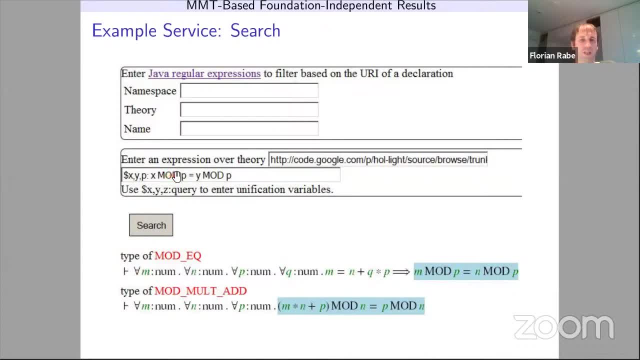 where mod is one of the constants in one of the series. in the whole line light library We have a generic search engine that does unification, substitution, tree indexing to find efficiently all terms anywhere in these huge libraries that unify with this and then shows you the results in the browser. These are then two specific theorems in the 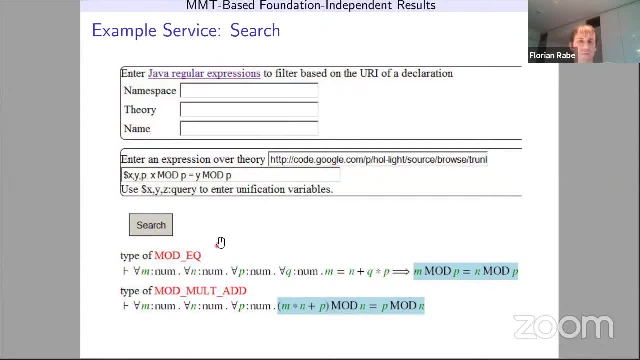 whole light library which were found A common. a current problem is: how can we do this in a way that we find results in multiple libraries. That's what I indicated earlier: that it's really hard to integrate these different libraries with each other. Just minor differences in. 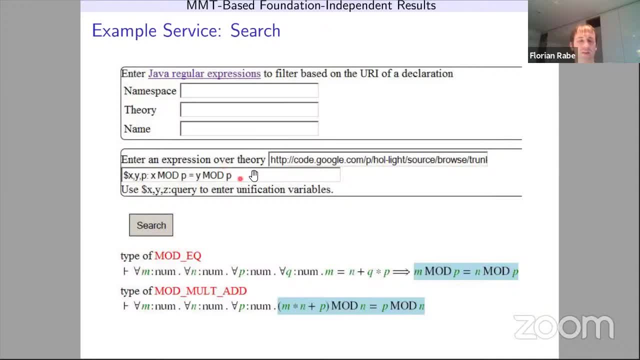 the type systems often have the effect that it becomes difficult to integrate them into one. to find results in multiple libraries With a modular operator it's probably still doable, but as soon as you have division, where systems disagree on how they treat division by zero, it can be tricky to find results across libraries. 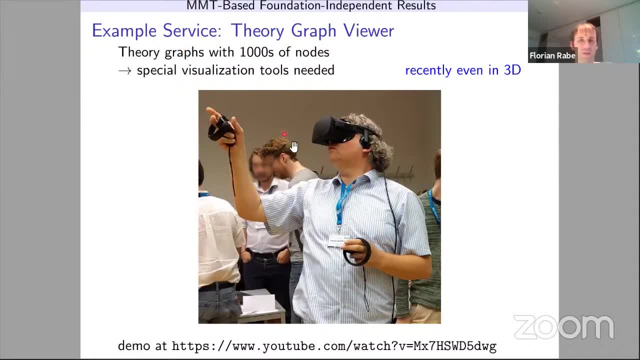 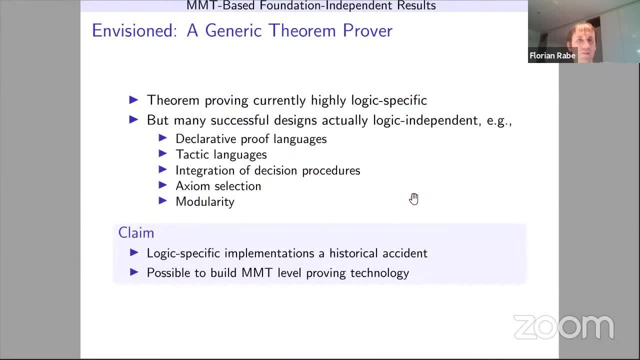 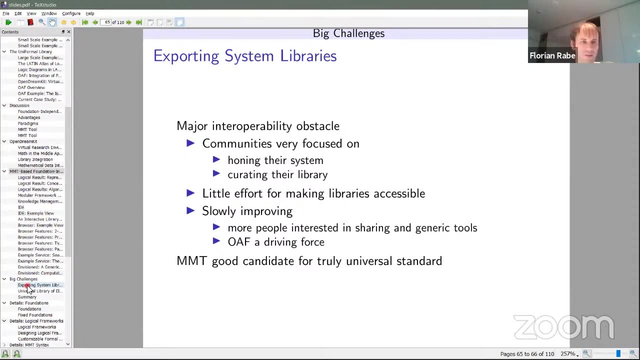 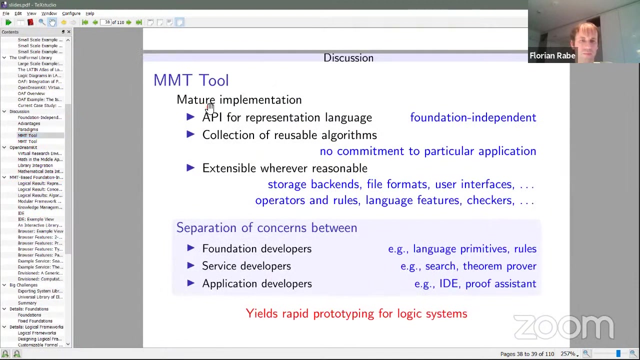 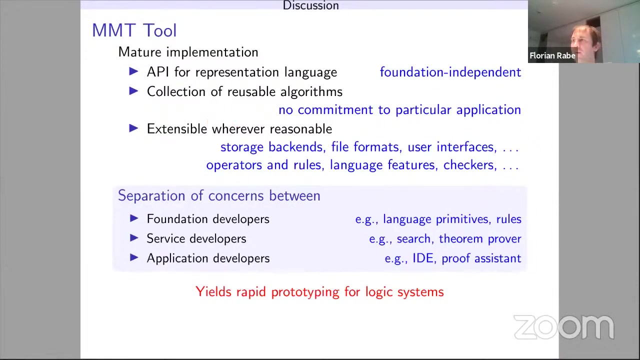 Our theory graphs became so big we started visualizing them in 3D. That was a big draw at conferences, And with that let me go to my conclusion slides. Okay, Okay, Okay. So MMT is quite maturely implemented by now. provides a foundation-independent way to represent. 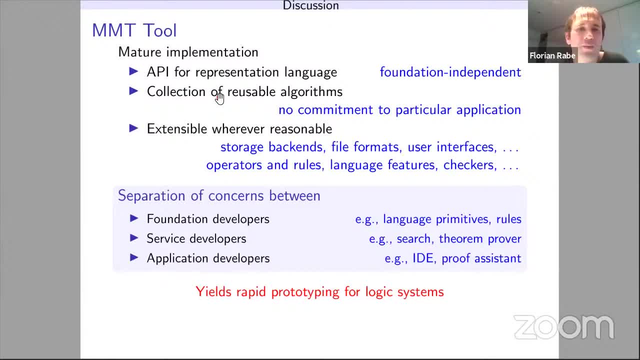 individual formal systems. It provides a growing collection of algorithms on top of that, such as parsing, type reconstruction or HTML generation, And it's also very easy to use. It's very easy to use, So MMT is quite maturely implemented by now- provides a foundation-independent way to represent. individual formal systems. It provides a growing collection of algorithms on top of that, such as parsing, type reconstruction or HTML generation, And it's also very easy to use. It provides a growing collection of algorithms on top of that, such as parsing, type reconstruction or HTML generation. 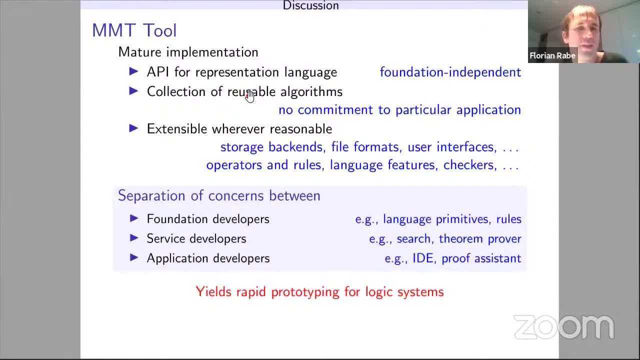 And that focuses on interactivity—interoperability—with other systems to determine whether system actions affect the execution goals of new algorithms during a problema or event. talking about ideas on technical process And extensibility, wherever I can figure out a way to make it extensible, to allow—to 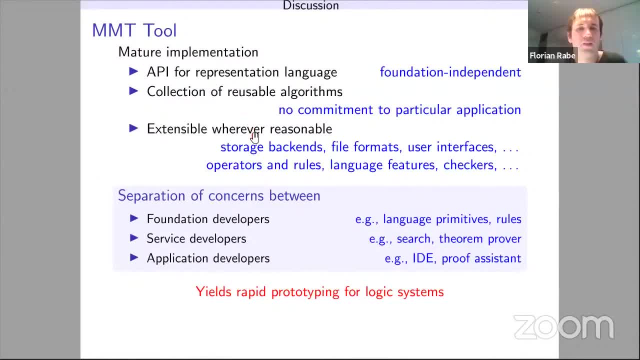 make it as easy as possible for users to write—other importers, other exporters, other kinds of logical rules- and write other importers, other exporters, other kinds of logical rules, And that leads to a very nice separation of concerns between the person who defines the. 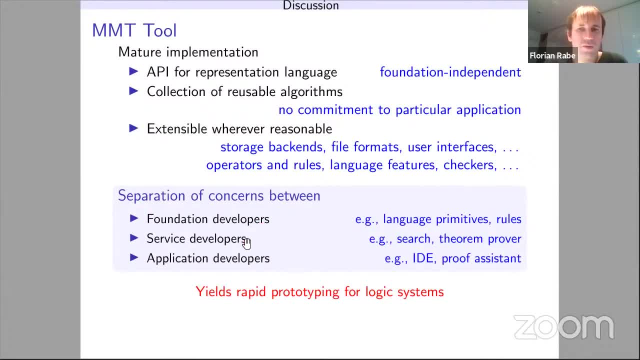 language and an expert in the application and exacerbating ideas in the implementation crash for language, the person who writes support services for that language and the application developers who use the system then to get other stuff done. I think I should stop here, because we said we stopped at 50 parts, right? 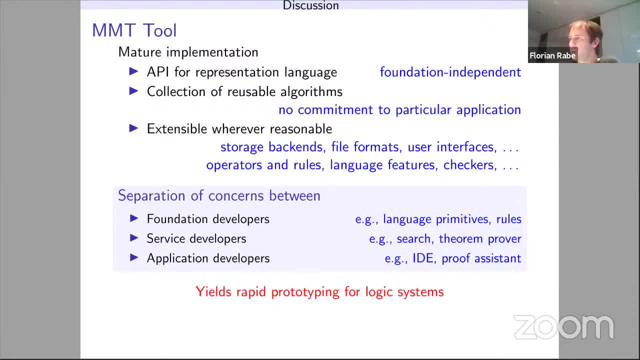 And this is as good a point as any if we want to have some room for questions. Let me check the chat again. One question I skipped: Have you done experiments to separate syntax-proof systems and models? I'm not entirely sure what you meant by that question. 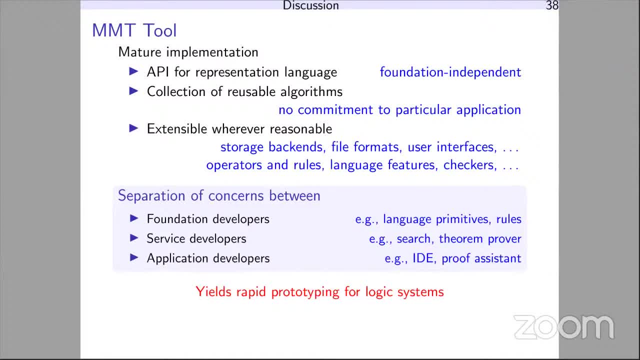 So maybe you can explain. Yeah, kind of, If you need the explanation of my question, I meant that it feels to me that the diagram is getting different levels confused, So kind of things like sorted first-order logic versus first-order logic, or I mean, can you get back to that MMT theory, the slide that had the picture? 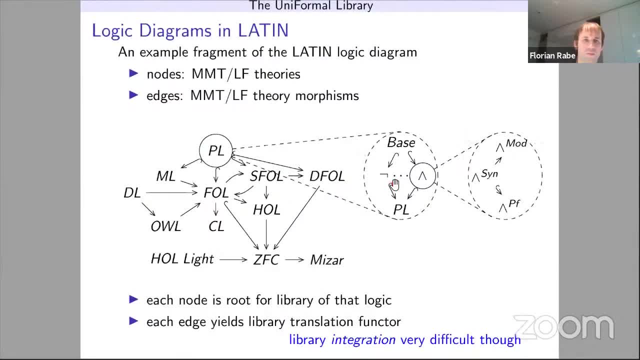 Mm-hmm. Yeah, Yeah, Yeah, Yeah, Yeah, Yeah, Yeah. This one, Yeah, You know, in this third little bubble there you have models, syntax and proof systems, right Yeah, And it seems to me that these things are on a different level from the difference between the. 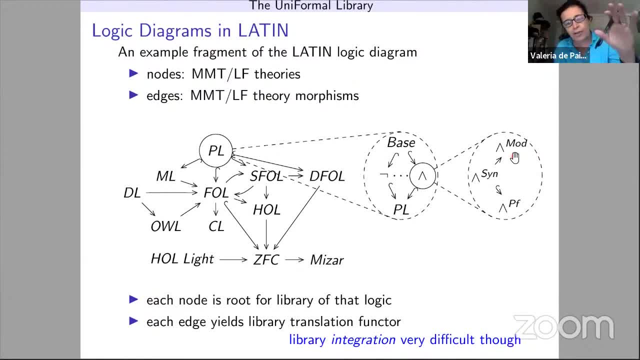 logic. So I was expecting you to do projections to each one of these things and to see, to try to look at them, to try to find some order on your big diagram. Actually, as far as MMT is concerned, there are just normal theories, So this one just happens to be a theory declaring proof rules. 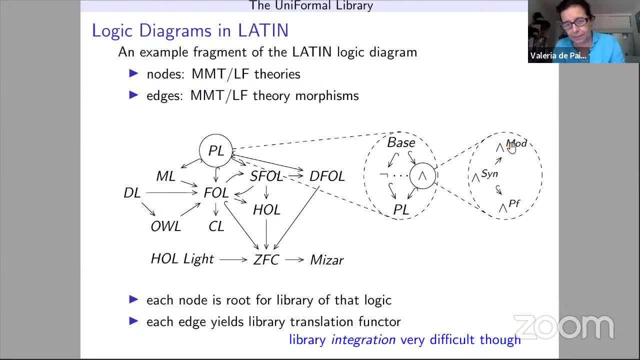 Right, And this one just happens to be a theory declaring the fundamentals you need in the model. But there is an orthogonality and it becomes a huge nuisance in practice, especially when you have to think about how to distribute all these theories into files. 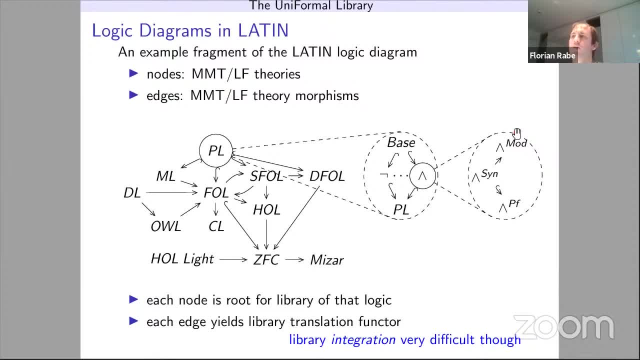 Like, do you want to put all the proof theory stuff in one folder, or do you put all the first-order logic stuff in one folder? Mm-hmm? Well, I was trying to say the opposite, right, Kind of not to put the first-order in one folder, but actually to put all the models together. 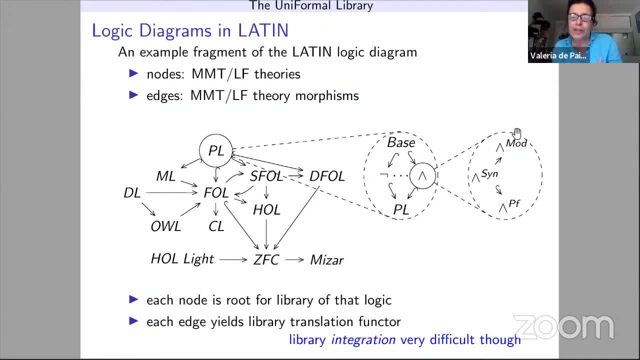 all the syntax together and all the, And especially the proof systems, because, you know, sequence systems are very different from Hilbert systems, which are very different from Pablo systems, Right? So that's the kind of experiments that I was asking if you had done. 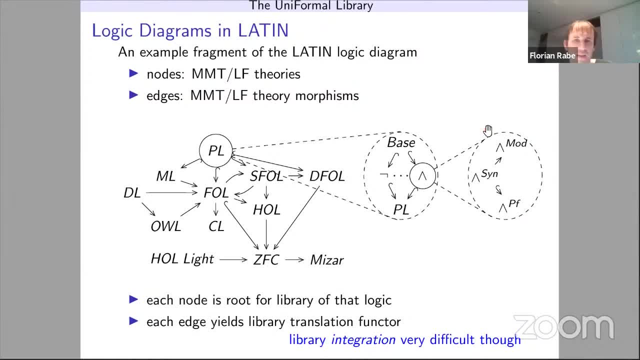 Yeah, So it gets even more Right, More messy in practice. And for all of these you have then the variant. What else can you prove if you happen to have classical logic, Or like the proof theory of conjunction? Well, conjunction is a bad example, but for every connective you usually have additional theorems. 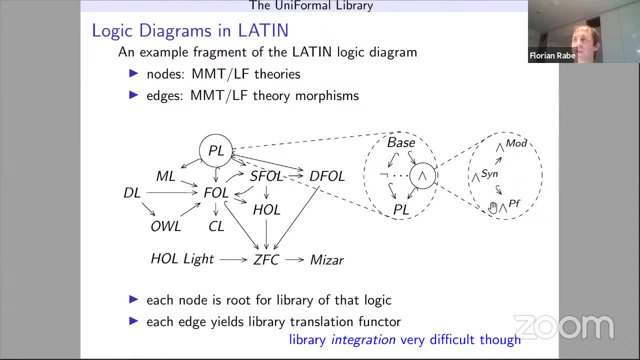 if you happen to be classical. So then the question is: where do you put all those theorems? Do you group all the classical theorems together, or do you group them with the respective Connective And then all of them have modal variants and 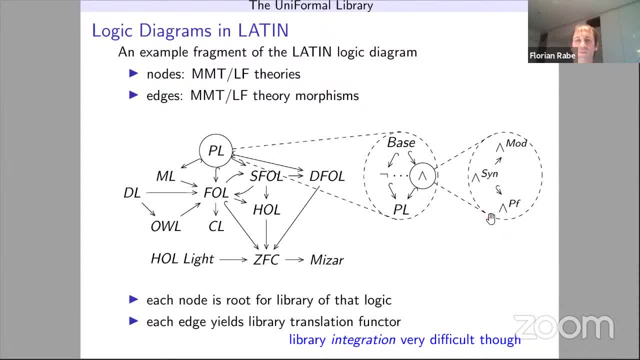 Yeah, So they are always separate in the sense that they're different theories in one huge diagram, But I don't really know how to best linearize them or how to best map them to this tree structure of a file system. Right, That was exactly the question: whether there is. 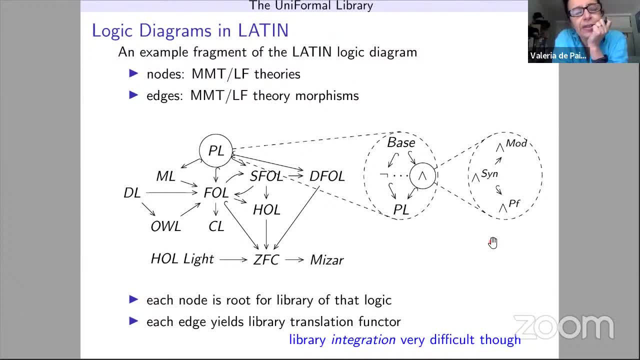 Any kind of lessons learned that you've got on how to linearize things after the event? No, And I think there's no good answer because different people in different situations will need different linearizations. Right, But you know, if you kind of have this whole messy thing, you presumably can do different. 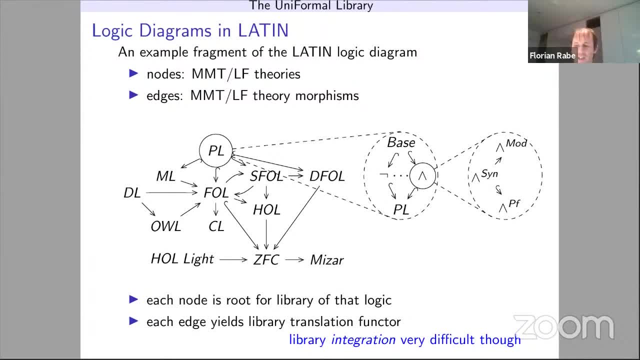 projections in different directions, Right. But you know, if you kind of have this whole messy thing, you presumably can do different projections in different directions, Right. We have those projections in the, So Michael usually likes to call them guided tours. 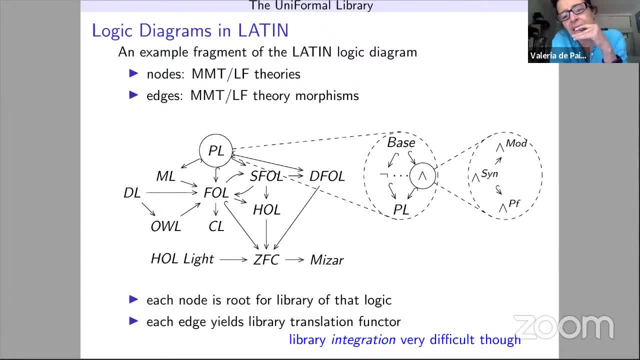 where you say one theory and then the system gives you the sub-diagram that has exactly the material you need to understand that one theorem That works reasonably well. Michael uses it in his lecture notes a lot- Right If he wants to introduce a particular concept. 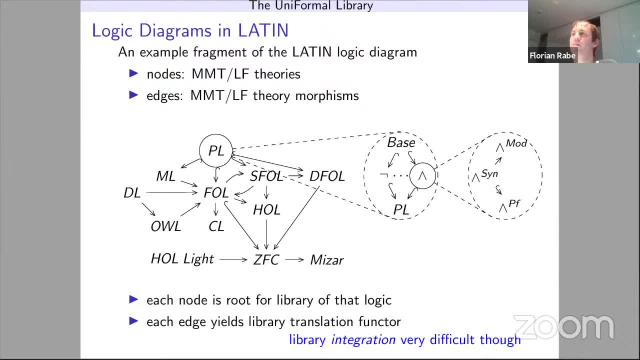 he can generate the graph of all the prerequisites for that concept- Cool. But that usually requires quite a lot of infrastructure on top. that has to work because the user isn't working with the original source files anymore, but with the view onto the source files generated by the system. 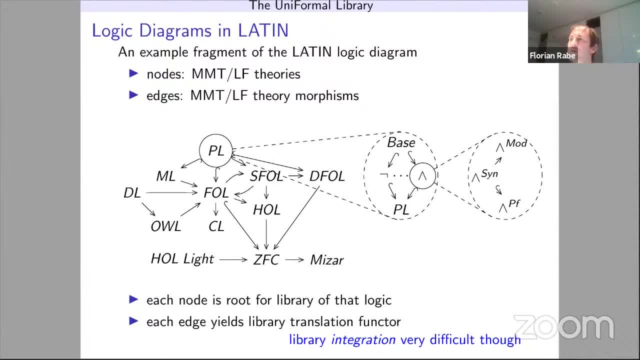 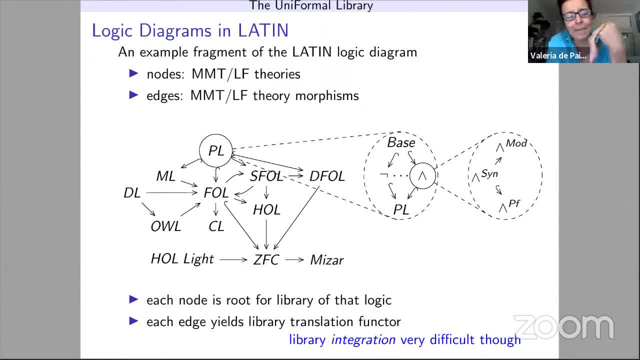 So I mean, I think the question I had, I mean this was an instantiation of a more general question, because you say, down there in blue library integration is very difficult though. So what I was kind of trying to ask more in general is: 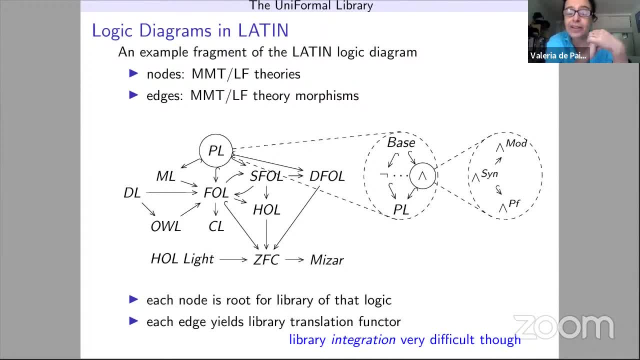 how do we kind of: Do you have at the moment any great theory of how you're going to try to improve on library integration and library decomposition? I mean, I assume that library integration you mean picking up the PVS library and putting together with the Hall-Light library. 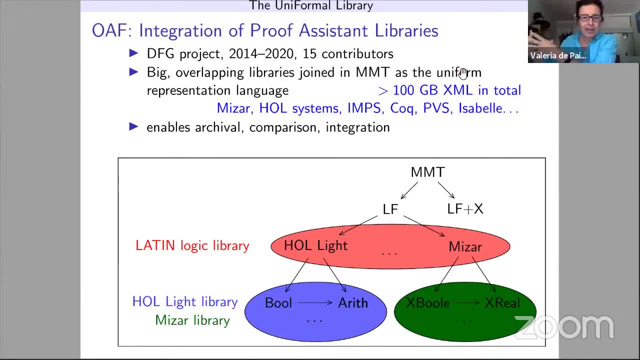 Right, That would be one nice thing to do. yeah, On the other hand, I also think that we want to kind of do decompositions right. Kind of you know, here you're decomposing, saying Hall-Light is different from MISA. 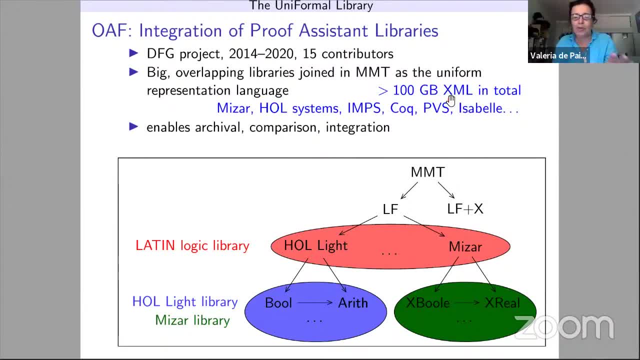 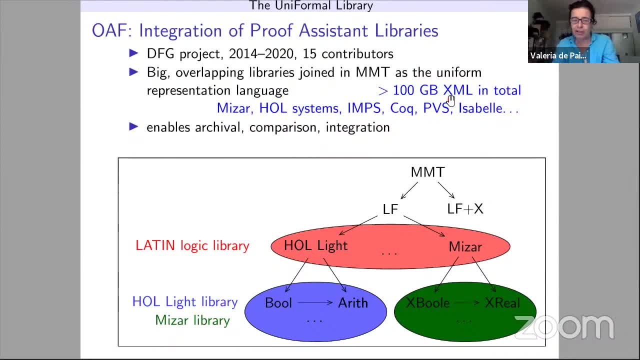 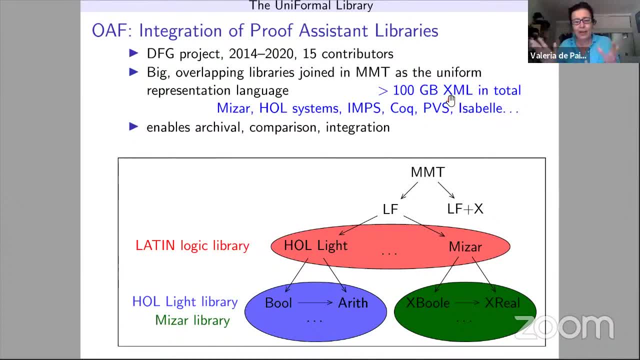 Every single one of those is Every single one of those. so the question is- And maybe someone will come and say, no, that's not the right way of separating It's. you know, they both have a bullion saying so it kind of that's how I want to separate. 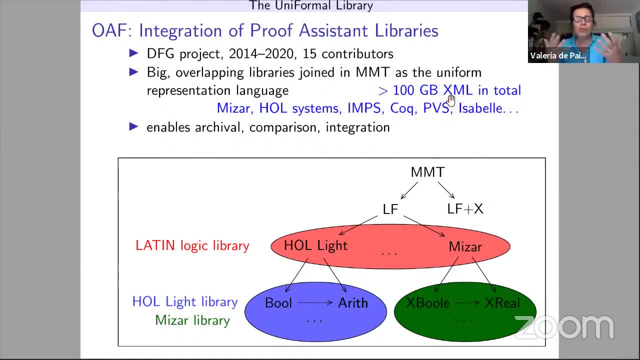 So whether you have any new big insights along these lines of integrating and decomposing those libraries, lots of insights, lots of experiments, but no ready to use instructions for how you can do it like. let me give you just one data point: already in coq alone, there's like i don't know, five or 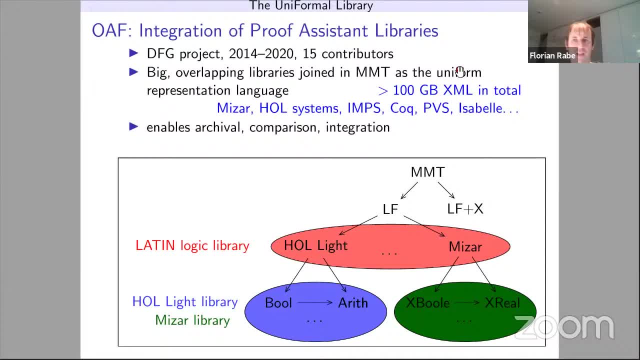 ten different versions of the real numbers. so it's not even just integrating across libraries. even within the library it's a mess, and the maintainers of each library are struggling to have some semblance of order in there. the one thing i can say is systems should strive to follow the little series approach. 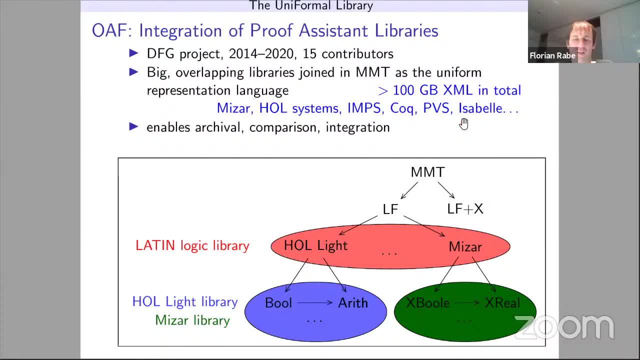 of formalizing every concept in, you know, in the smallest context in which it makes sense. unfortunately, systems don't do that in practice. so it's a big proof assistance. actually, the reason why we have ims on this list, even though it's not a big proof assistance, is it's the one system that 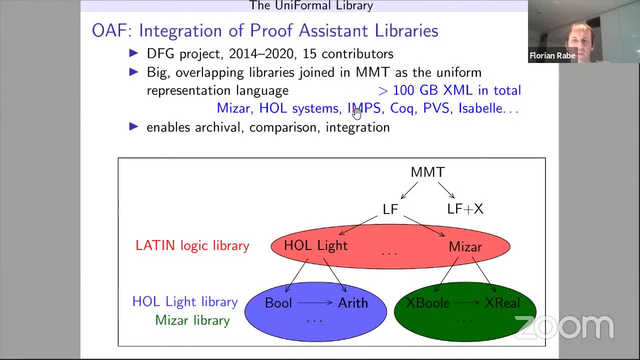 systematically uses little series: coq, pvs and isabel supported in principle but then in practice it's not used that much. isabel type classes are used a bit. pvs does use some modularity for the algebraic hierarchy in similar situations but overall it's not used enough i would say in all of these systems. 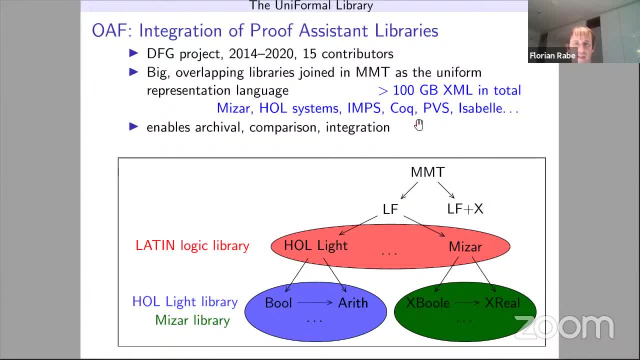 and that means if you just take any crm from any one of these libraries, the dependency that you need will be everything in that systems library, down to the foundations, and just disentangling that to say, hey, this theorem about arithmetic really only depends on the piano axioms. 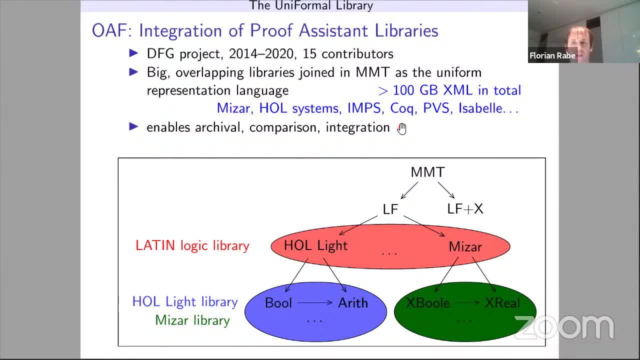 and we can abstract that away. then we map the piano axioms to some other proof of system and we can transport that theorem over. and we can abstract that away. then we map the piano axioms to some other proof of system and we can transport that theorem over. 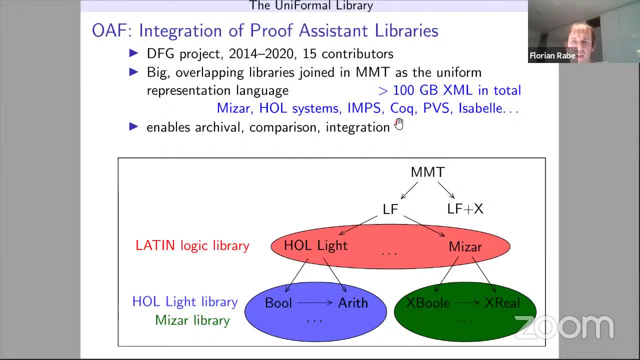 most systems just don't offer that kind of infrastructure. so very often the best method would be to go into these various libraries and restructure them systematically to have more modularity in the libraries. the jill doex group in around deducty they've actually kind of done that a bit for a tiny arithmetics library. 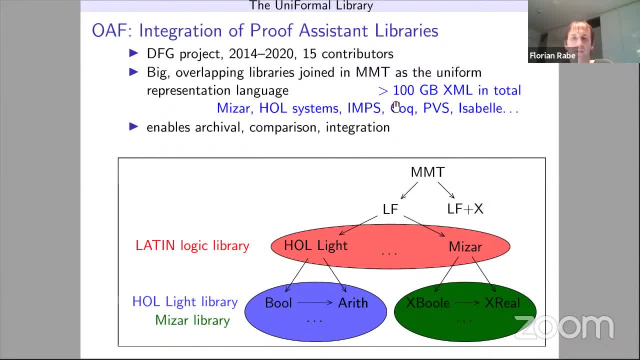 they've actually kind of done that a bit for a tiny arithmetics library, and then they were able to port that one into the different theorem provers. so as an experiment it shows the method, but it just we don't know how to scale it up to the. 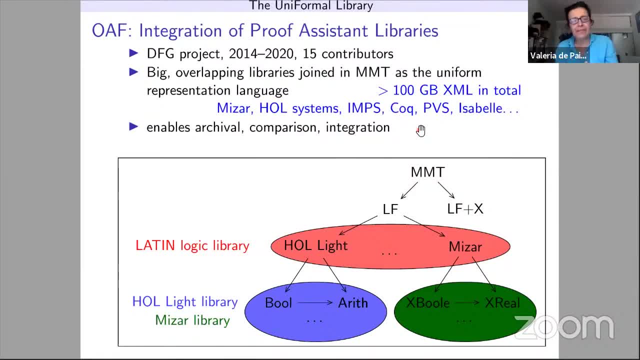 huge libraries that we have. well, thank you that. that that's very helpful. thank you, yeah, let me um interrupt. i think we should thank florian. uh, everyone can unmute and clap or just put the symbol. um thanks for the great talk, florian, and i think we will cut the live stream and then anyone who wants to stay and ask. 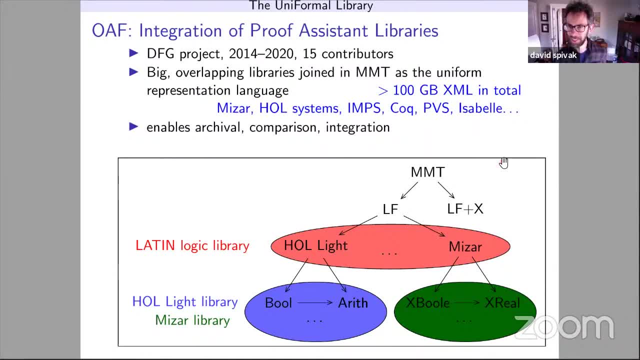 informal questions. um, please feel free. so thanks again. okay, great thanks for having.